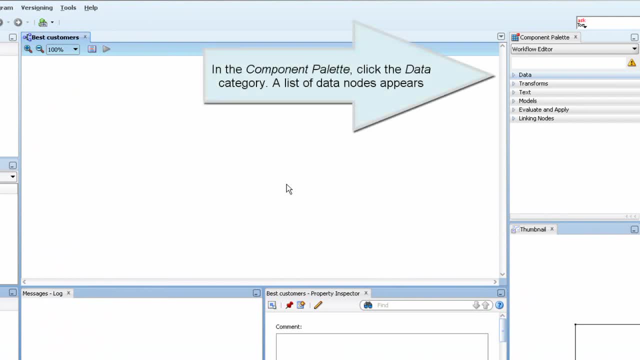 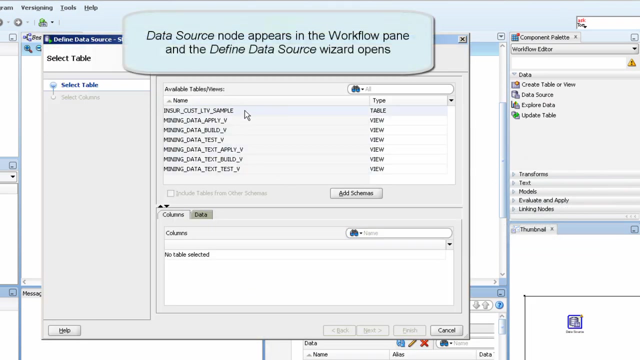 In the component palette, click the data category. A list of data nodes appears. Drag and drop the data source node onto the Workflow pane. Data source node appears in the Workflow pane and the defined data source wizard opens. Select, Ensure, Cust, LTV. Sample from the Available Tables: Views list: 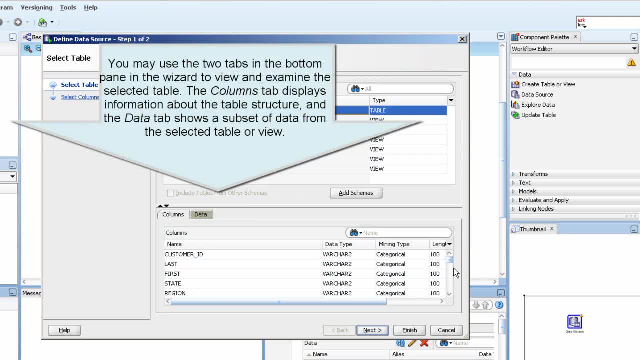 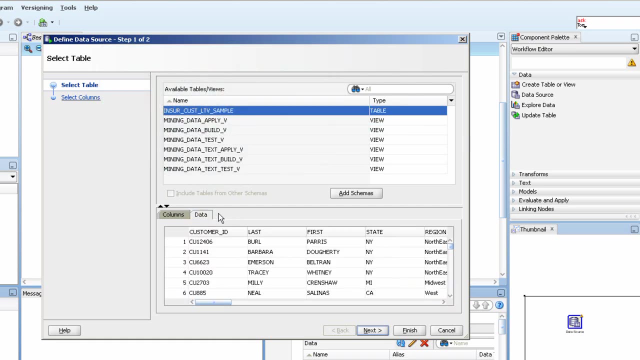 Select Ensure Cust LTV Sample from the Available Tables Views list. Add employees: Click Cust LTV Sample from the Available Download. dia45m latest file. In thewhere Portacle lots are matched with good site. click OK, Click OK, Click OK. 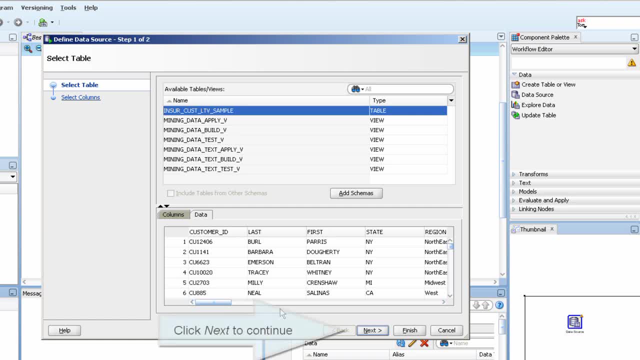 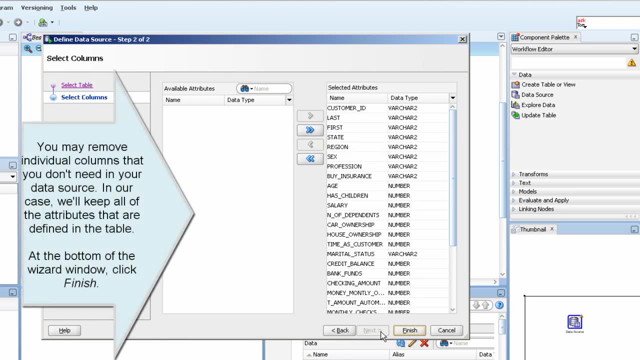 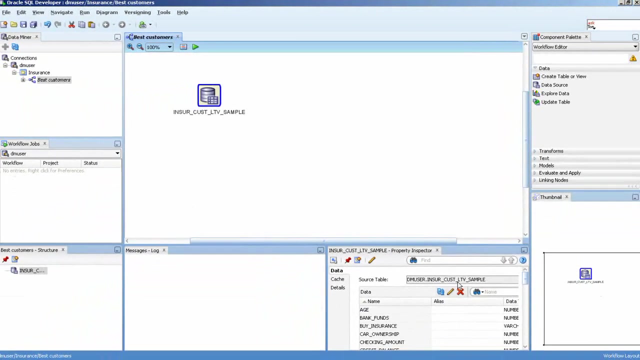 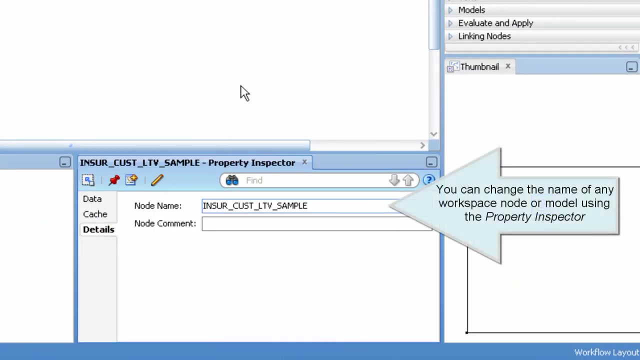 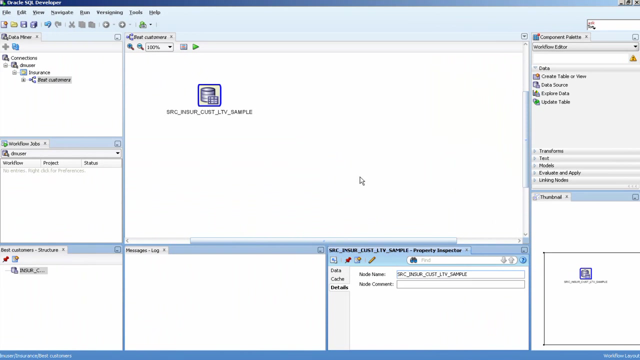 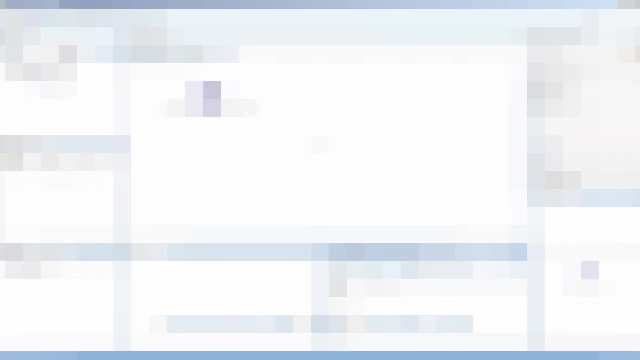 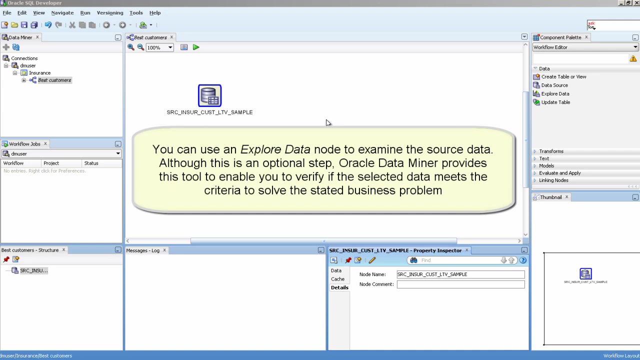 Click Next to continue. The data source node name is updated with the selected table name and the properties associated with the node are displayed in the property inspector. You can change the name of any workspace, node or model using the property inspector. Define the data. 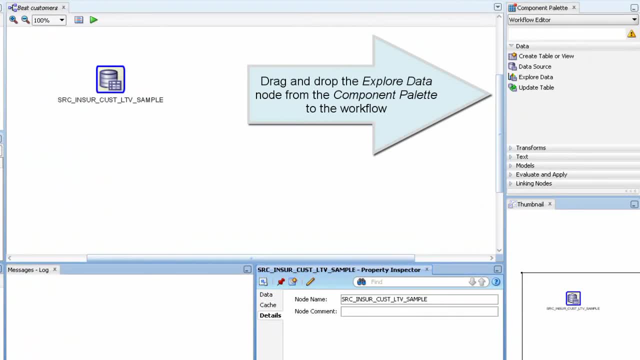 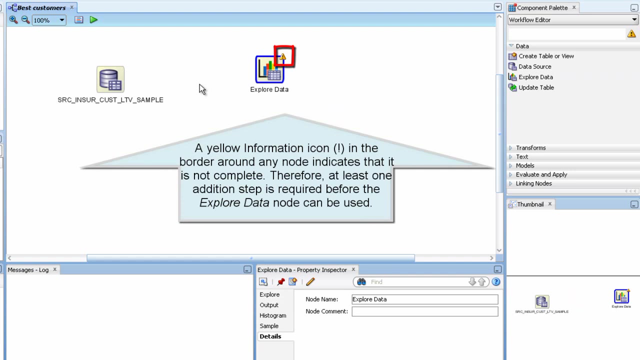 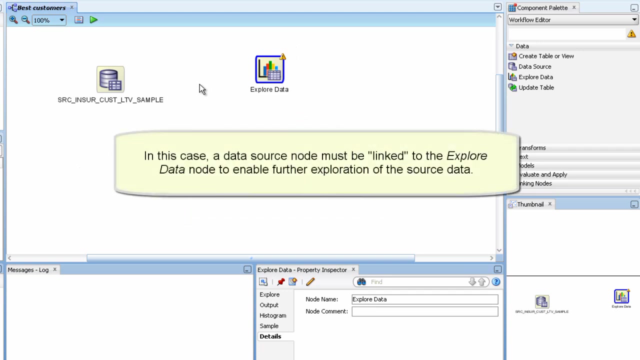 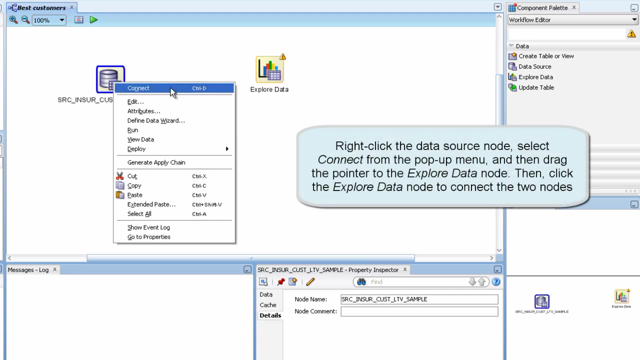 Drag and drop the Explore Data node from the component palette to the workflow. Next, Next, Next, Next, Next, Next. Right-click the data source node, select Connect from the pop-up menu and then drag the pointer to the Explore Data node. 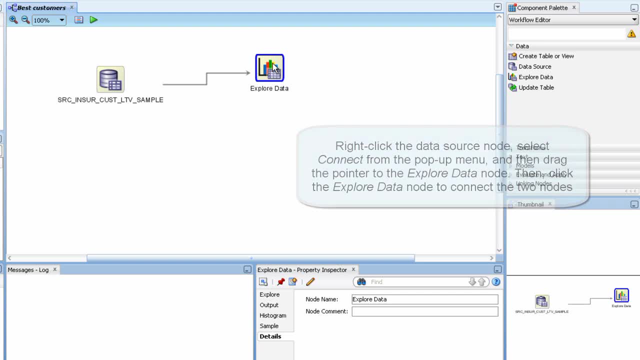 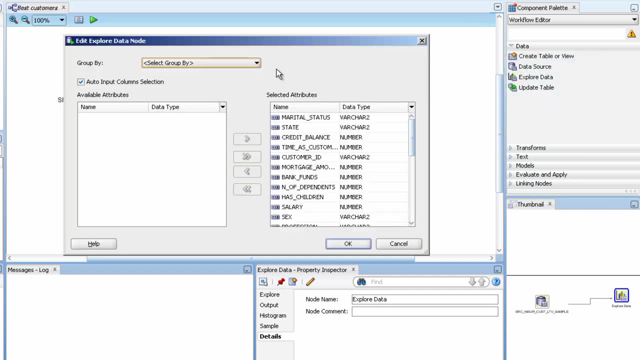 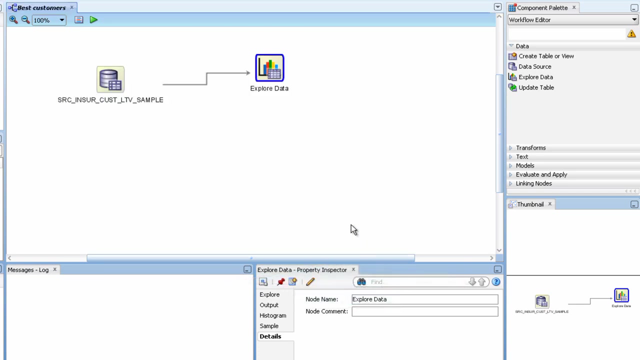 Then click the Explore Data node to connect the two nodes. Double-click the Explore Data node to connect the two nodes. Explore data node to display the select attributes window In the group buy list. select the buy insurance attribute. Then click OK. 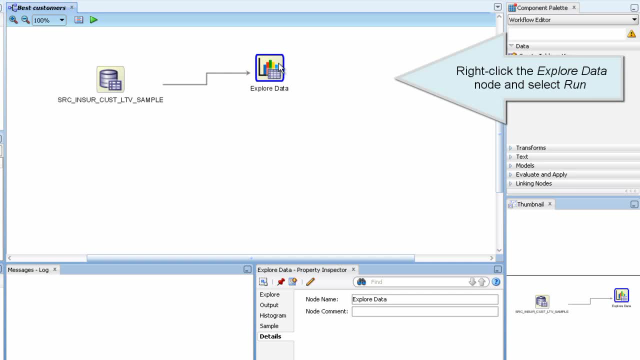 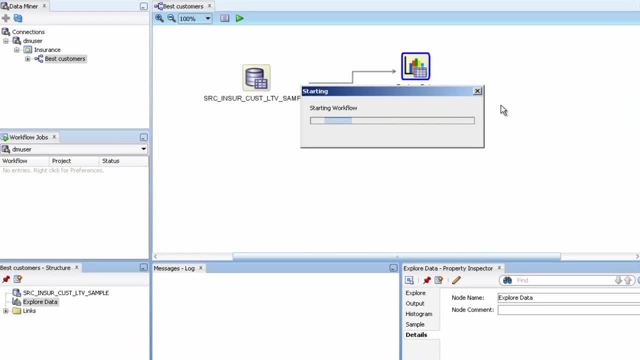 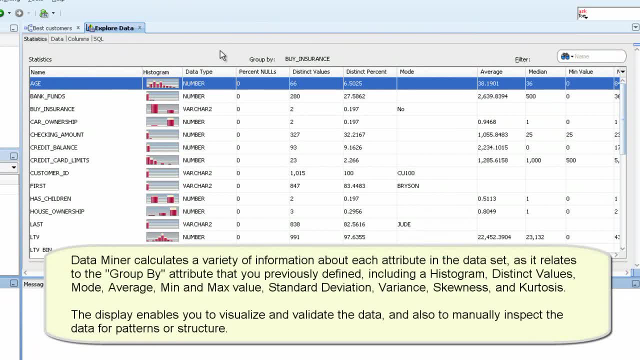 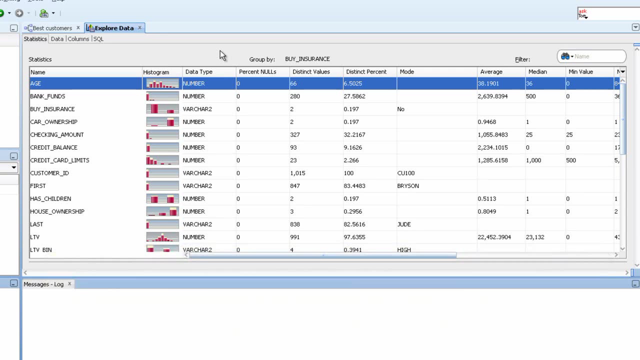 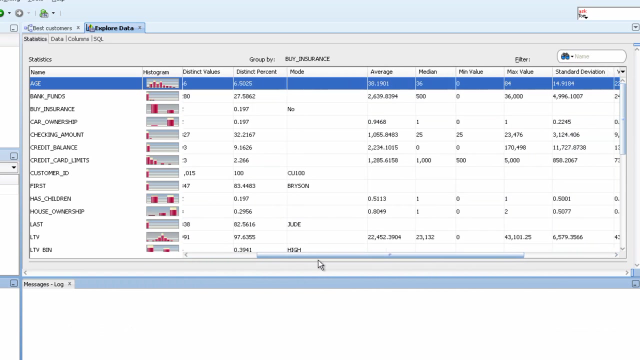 When the update is complete, the data source and explore data nodes show a green checkmark in the borders. When the update is complete, the data source and explore data nodes show a green checkmark in the borders. When the update is complete, the data source and explore data nodes show a green checkmark in the borders. 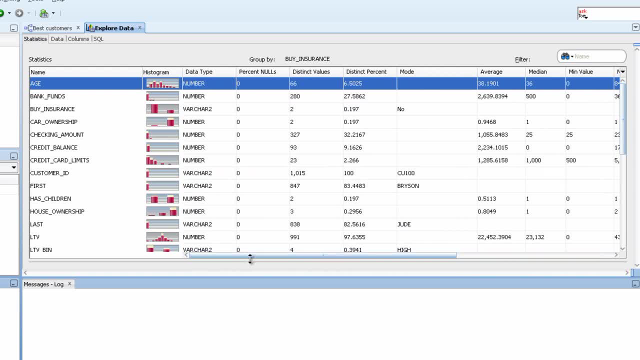 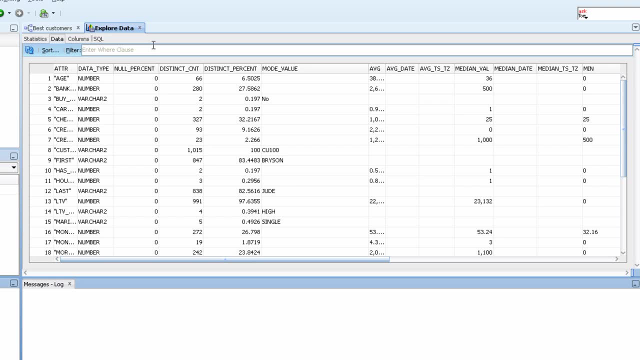 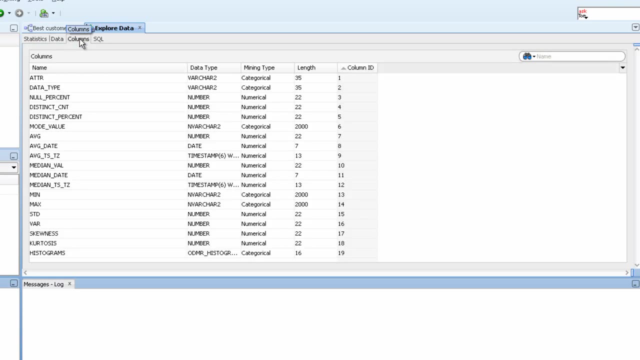 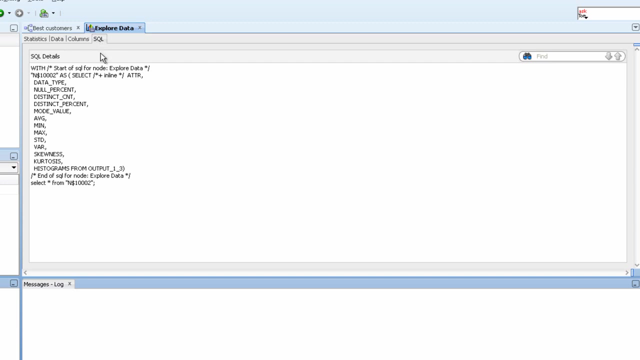 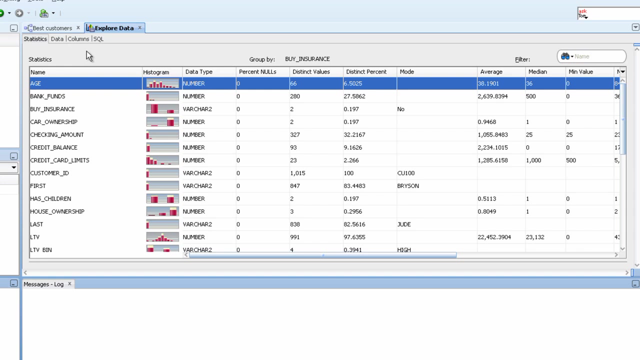 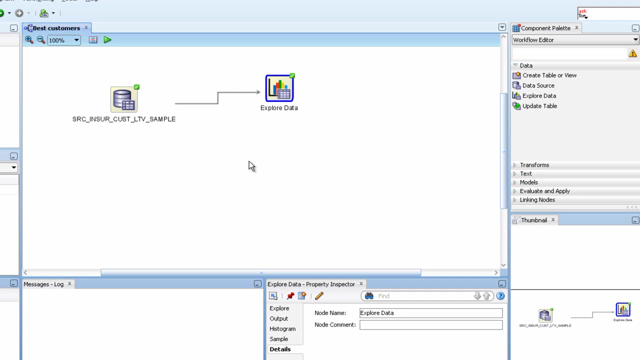 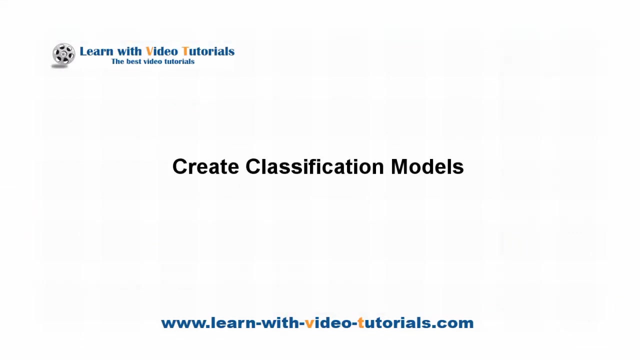 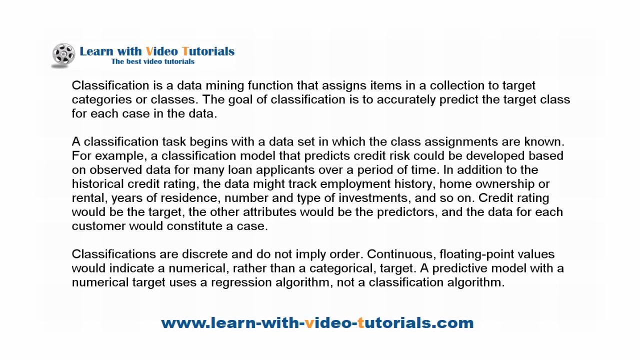 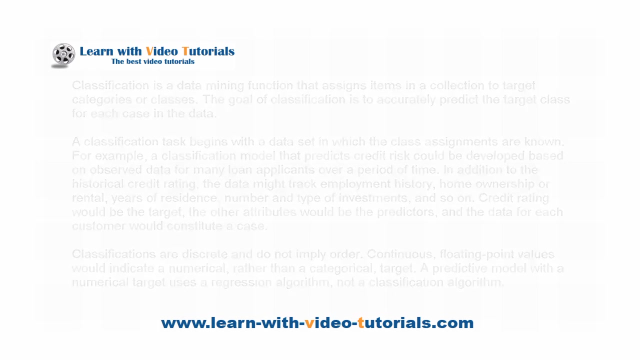 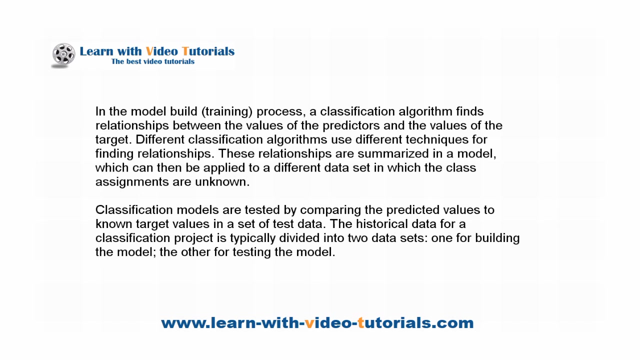 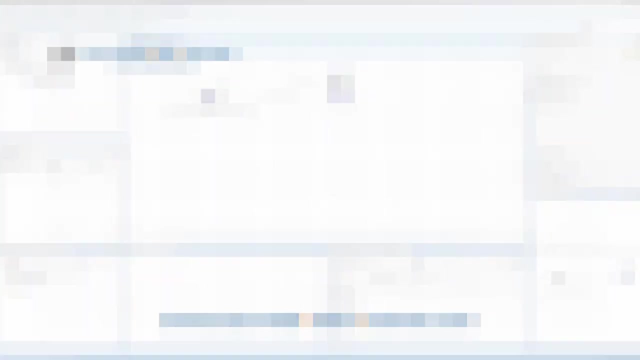 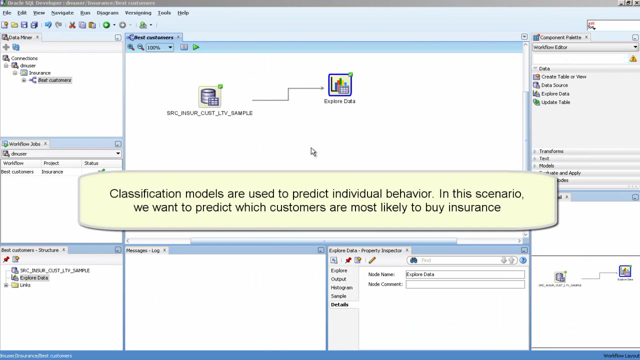 When the update is complete, the data source and explore datacore data nodes show a green checkmark in the borders. Thank you, Create classification models. Create classification models. Classification models are used to predict individual behavior. In this scenario, we want to predict which customers are most likely to buy insurance. 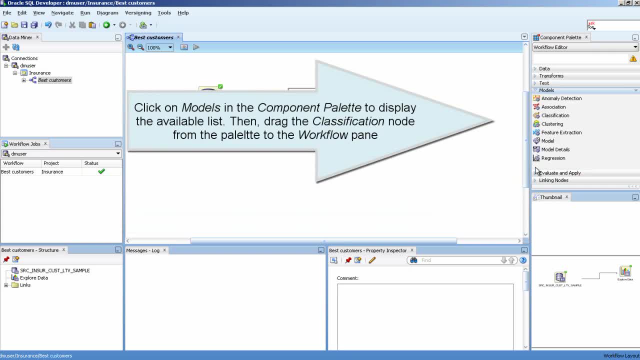 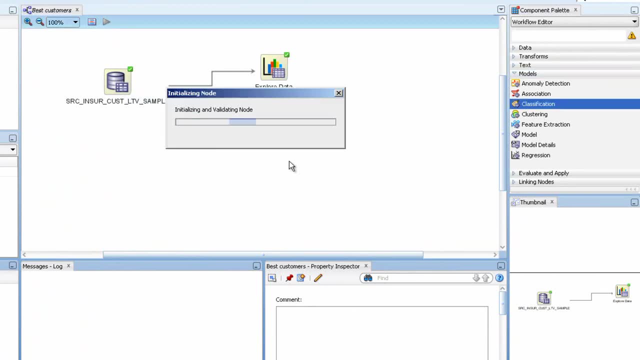 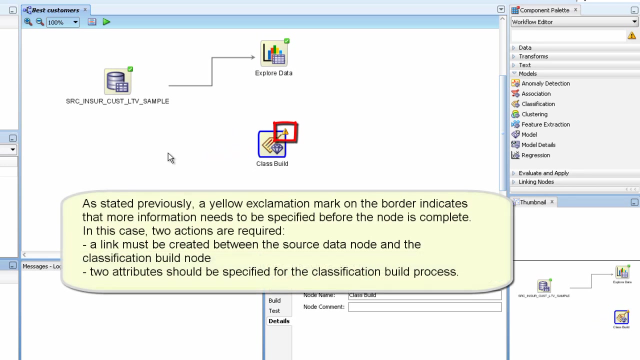 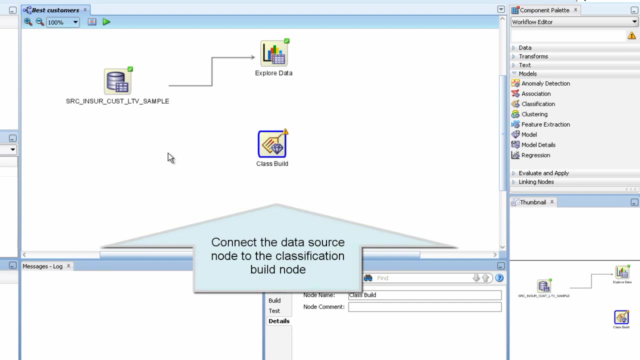 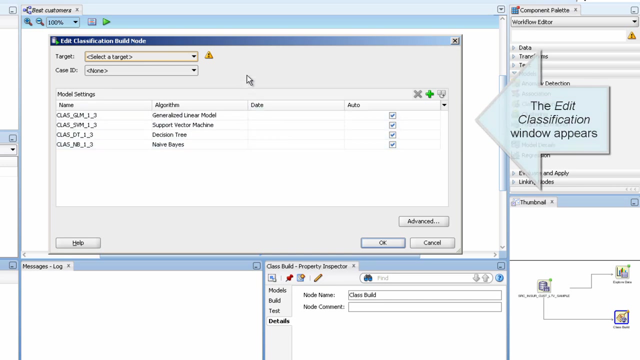 Click on models in the component palette to display the available list. Then drag the classification node from the palette to the workflow pane. Connect the data source node to the classification build node. The edit classification window appears. A yellow indicator is displayed next to the target field. 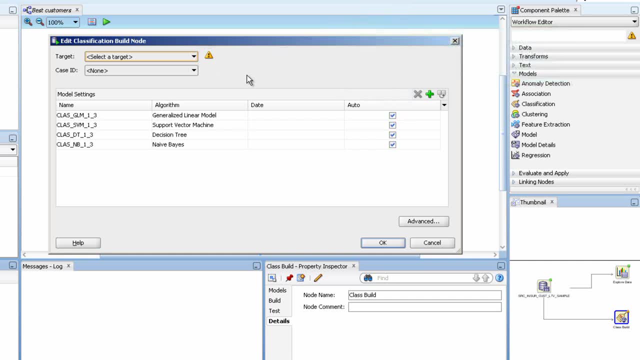 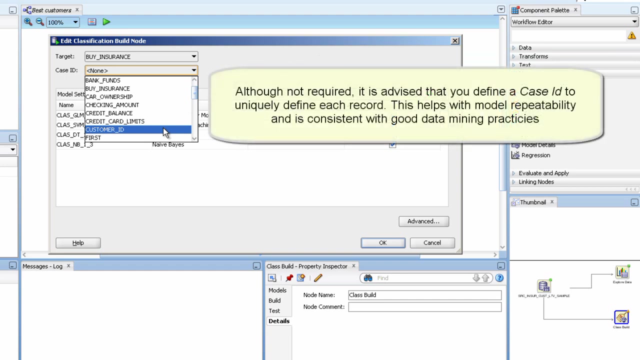 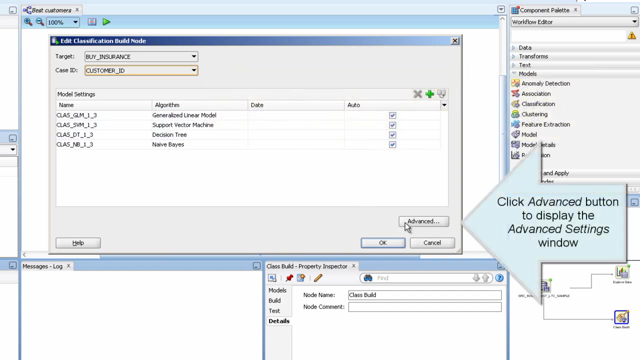 This means that an attribute must be selected for this item. Select by insurance as the target attribute. Select customer ID as the CASID attribute. Click Advanced button to display the Advanced settings window. Click Advanced button to display the Advanced settings window. Click Advanced button to display the Advanced settings window. 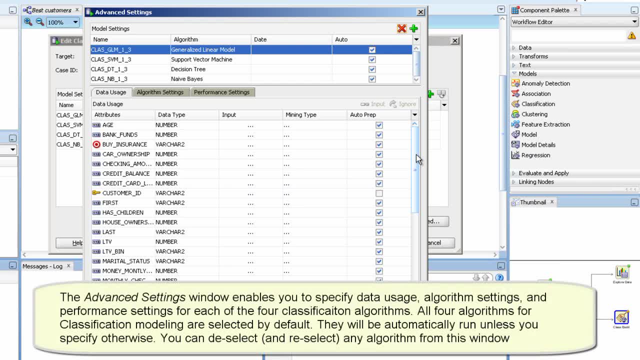 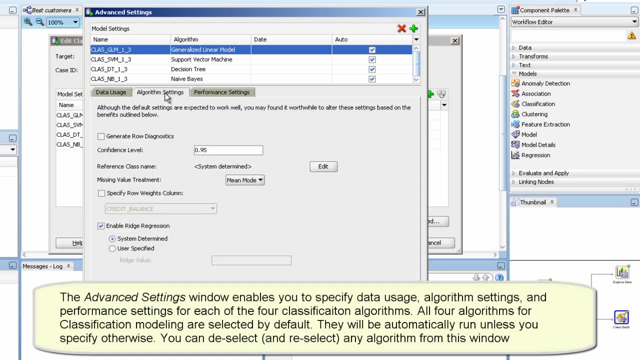 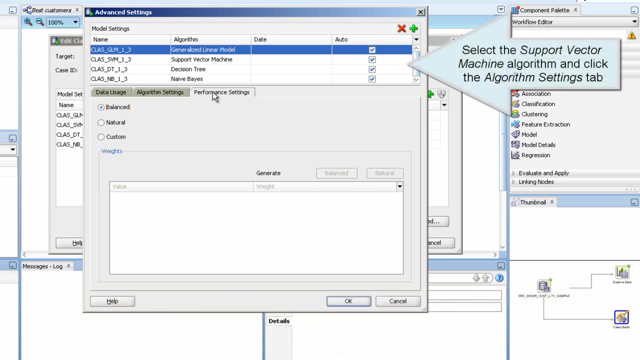 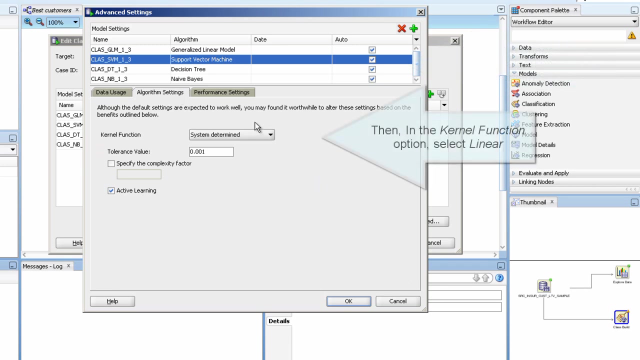 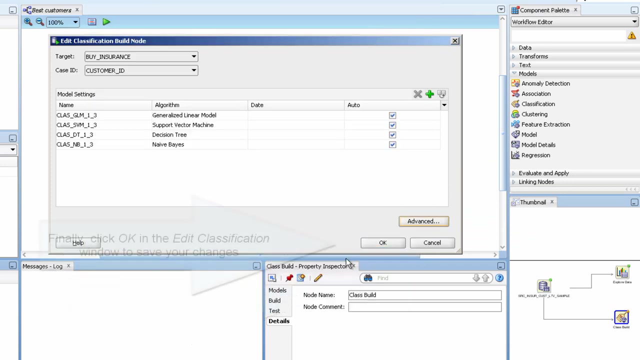 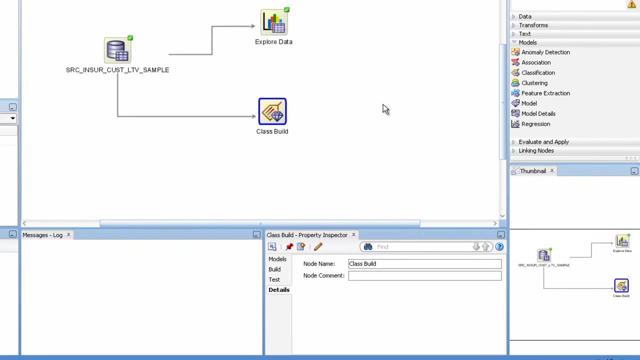 Select the Support Vector Machine algorithm and click the Algorithm Settings tab. Then in the Kernel Function option, select Linear. Click OK to save the SVM algorithm setting. Finally, click OK in the Edit Classification window to save your changes. In the Models tab of the Properties Inspector you can see the current status for each of the selected algorithms. 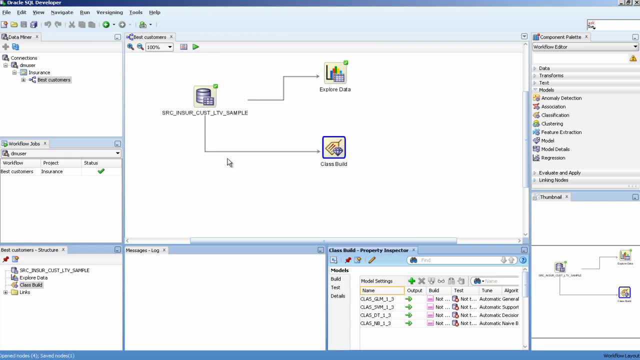 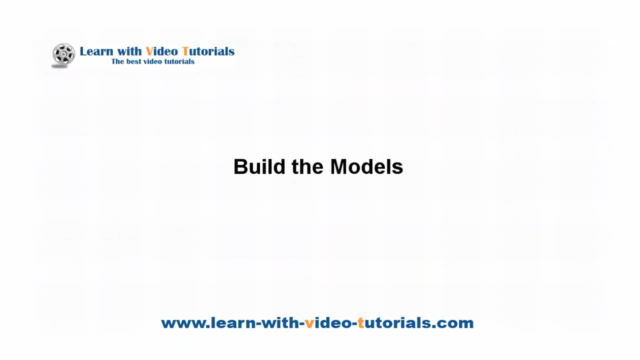 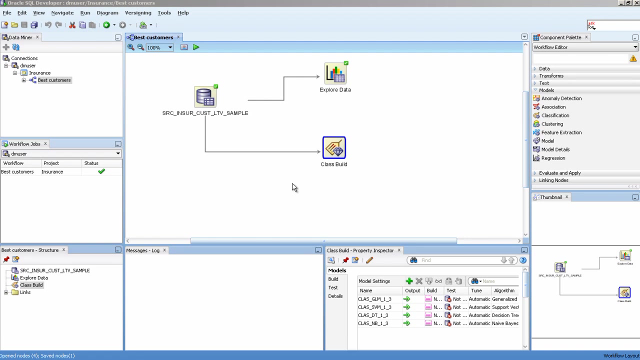 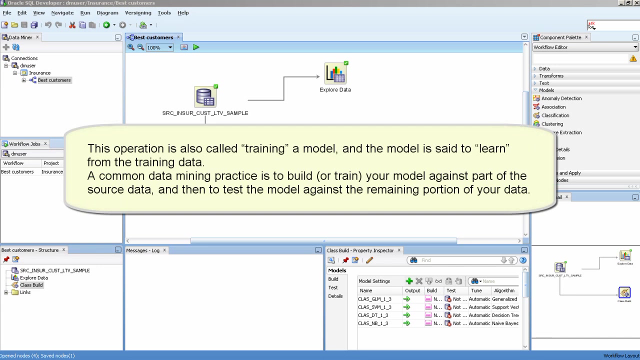 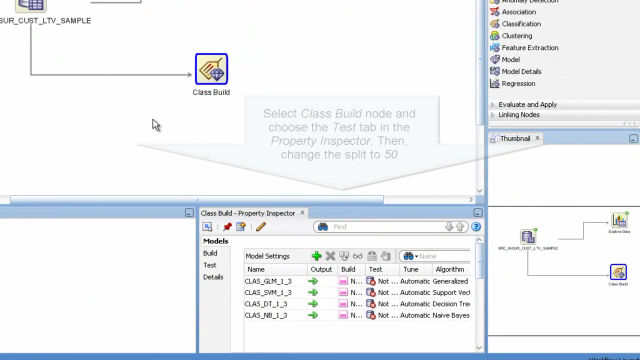 In the Models tab of the Properties Inspector, you can see the current status for each of the selected algorithms. Build the Models. In the Models tab of the Properties Inspector, you can see the current status for each of the selected algorithms. Select Class, Build node and choose the Test tab in the Property Inspector. 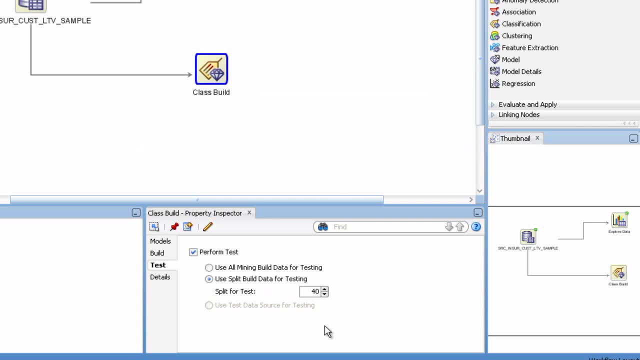 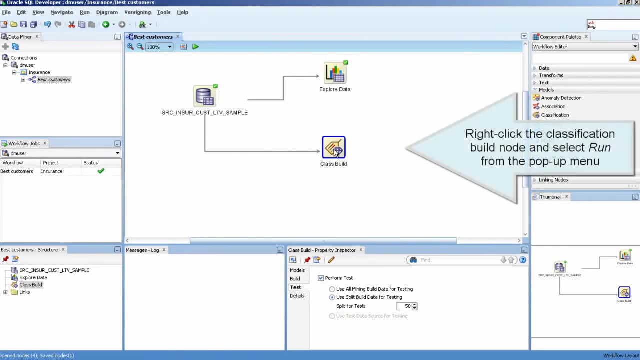 Then change the Split to 50.. In the Models tab of the Properties Inspector you can see the current status for each of the selected algorithms. Right-click the Classification Build node and select Run from the pop-up menu. When the node runs, it builds and tests all of the models that are defined in the node. 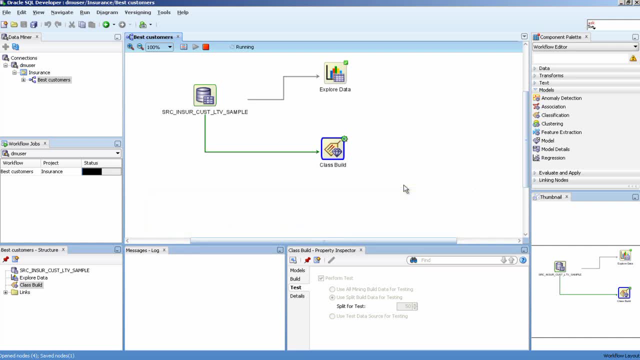 When the node runs, it builds and tests all of the models that are defined in the node. In the Models tab of the Properties Inspector you can see the current status and the current status of the model. It is good to add a new model. 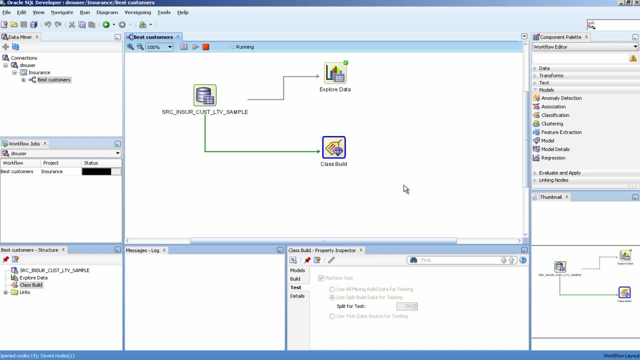 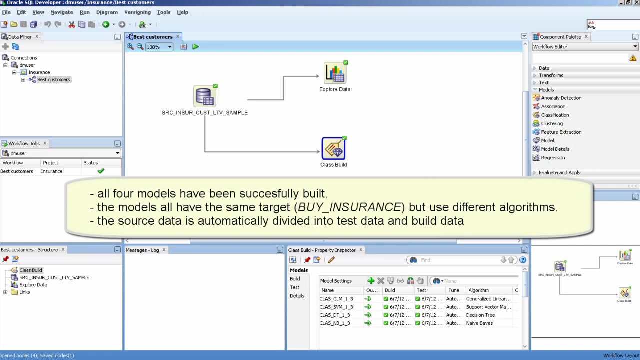 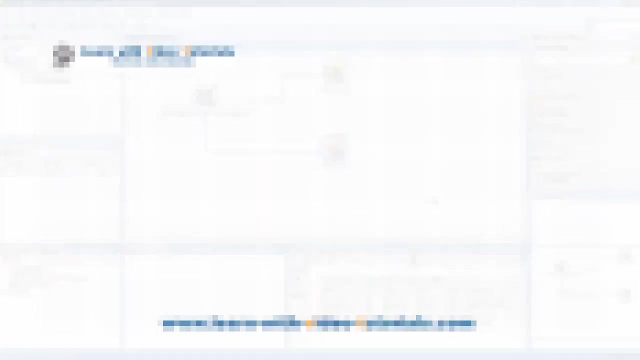 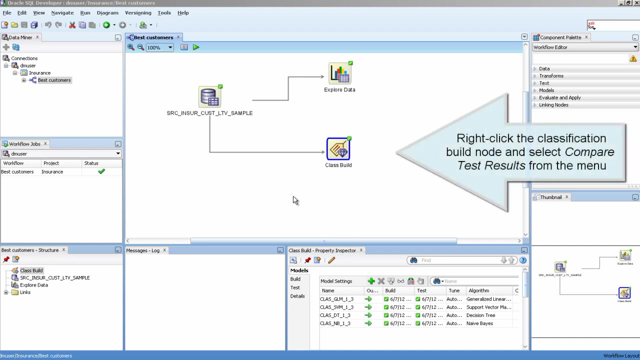 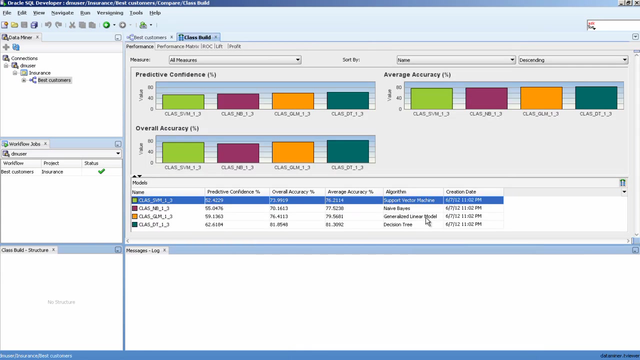 Let's start the build for theời. When the build is complete, the Status column displays a green checkmark. Select the Classification build node in the workflow and then choose the Models tab in the Property Inspector. Compare the models. Right-click the Classification build node and select Compare test results from the menu. 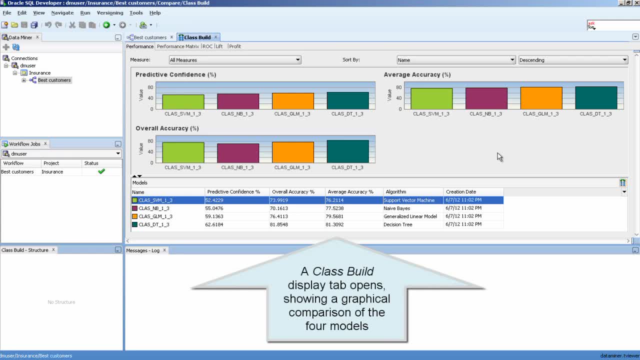 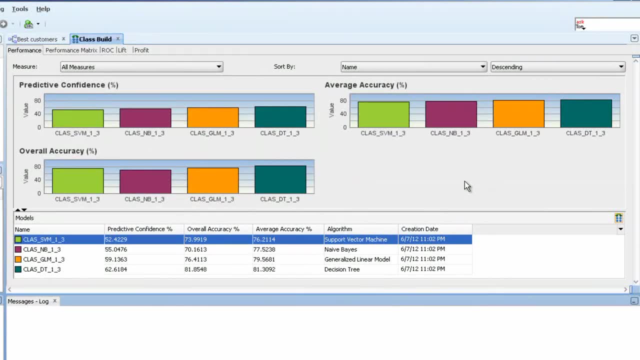 A Class build display tab opens showing a graphical comparison of the four models. OK. The comparison results include five tabs – Performance, Performance Matrix, ROC, Lift and Profit. The Performance tab provides numeric and graphical information for each model on predictive confidence. 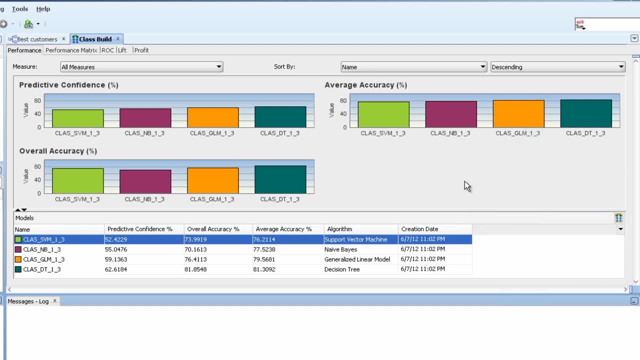 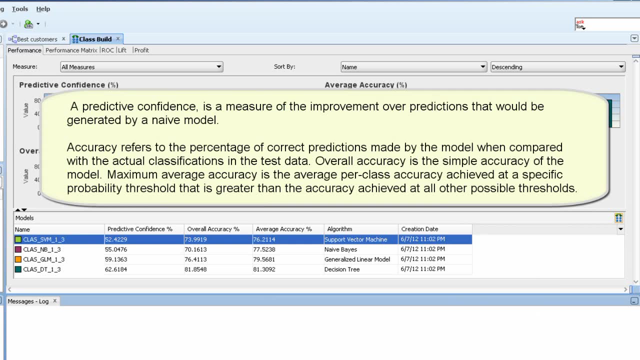 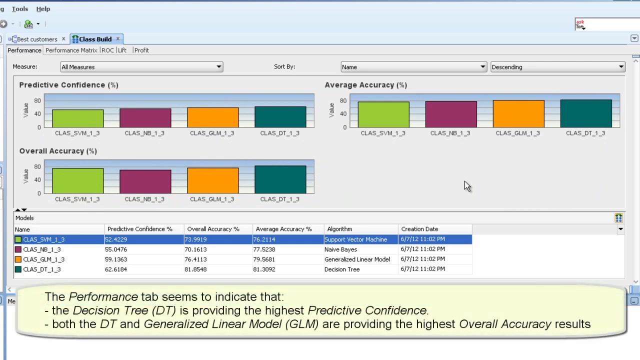 average accuracy and overall accuracy. In the 2D model, the performance report is set at the same value recorded by the PMV70.. The process will be the same for all models. When we align thealarys, the results appear on the monitor's columns as-is and the 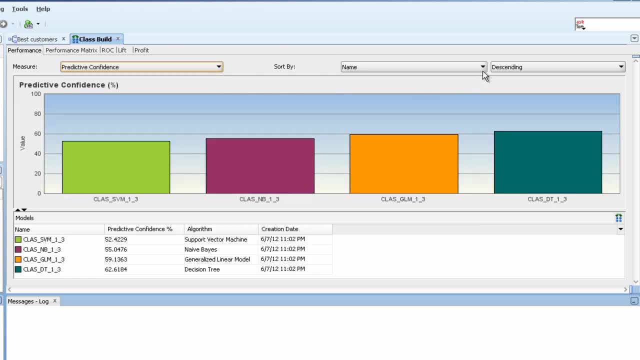 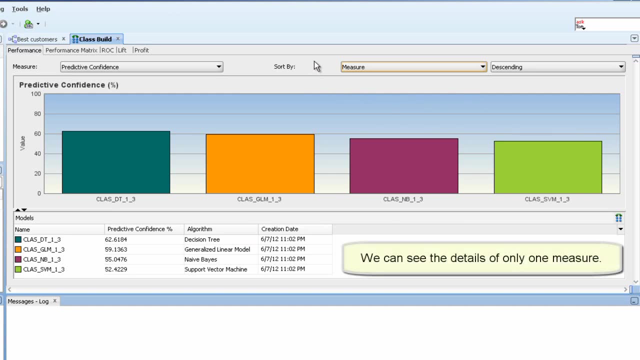 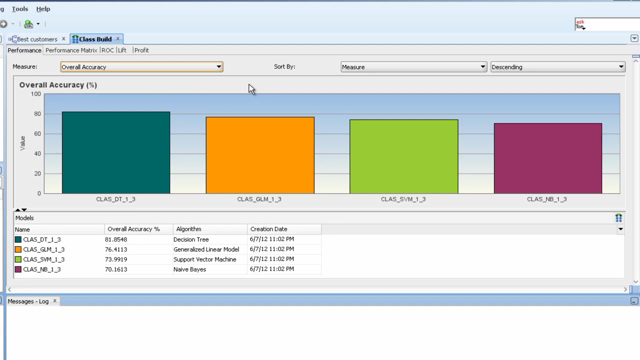 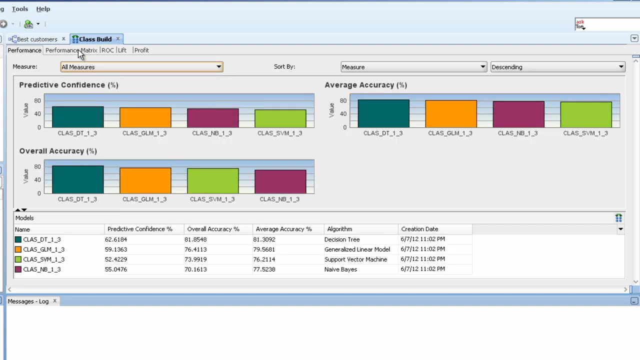 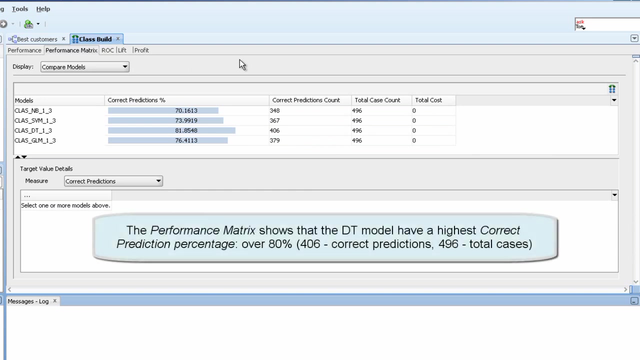 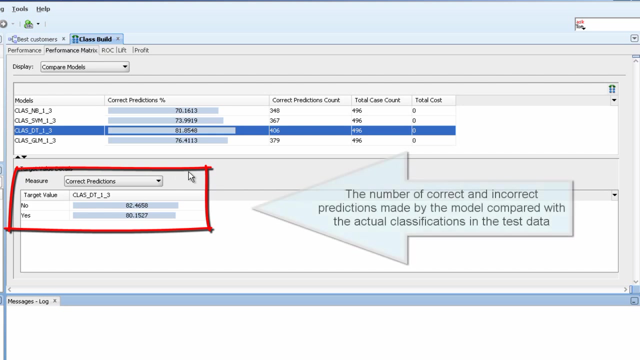 results are displayed View. View Eu consequential of results. overviewausociation reveals The results will be Ltd A т stall for new models and instruments. Benchmark Test block was defined as be set upon caramelization. Thank you, Thank you. Classifications in the test data. 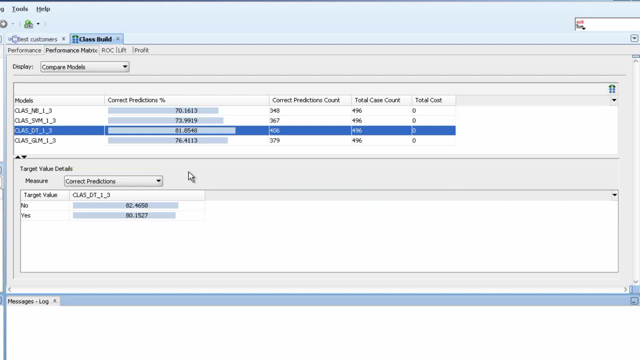 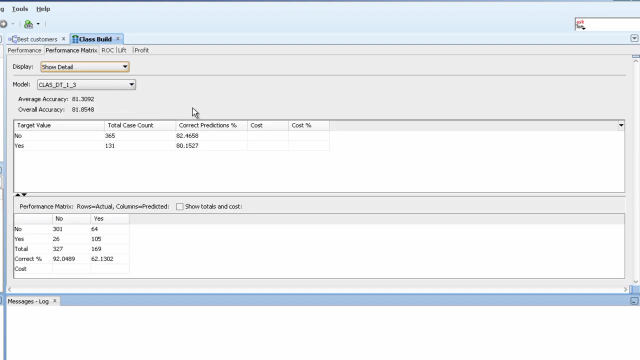 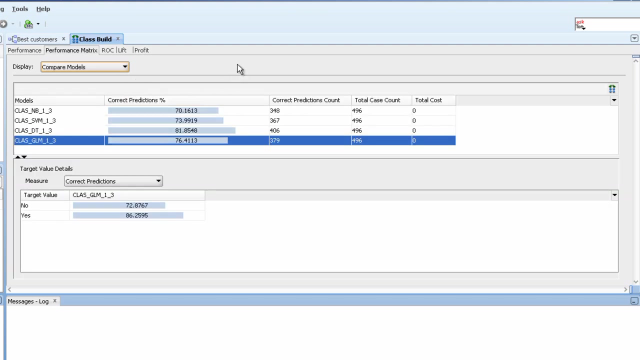 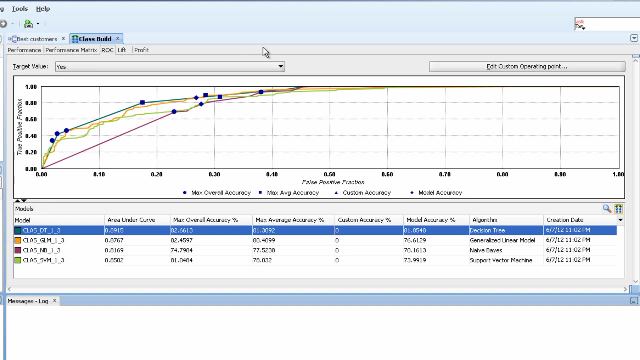 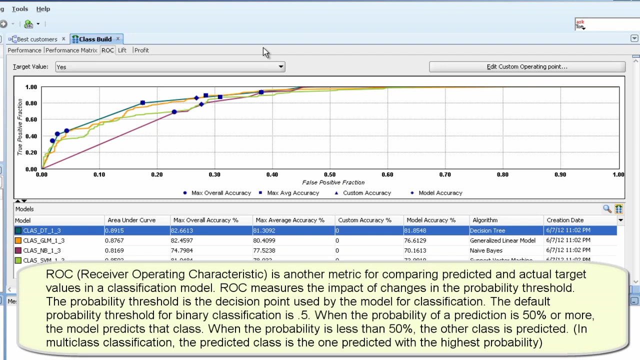 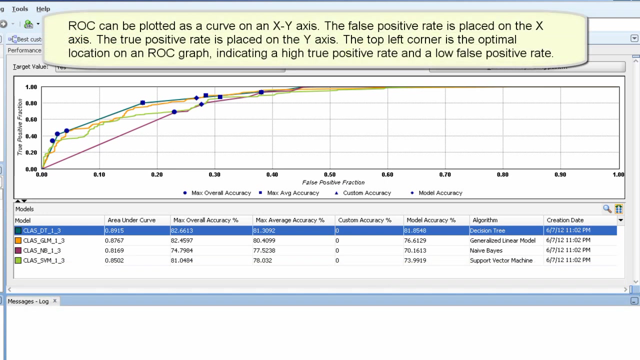 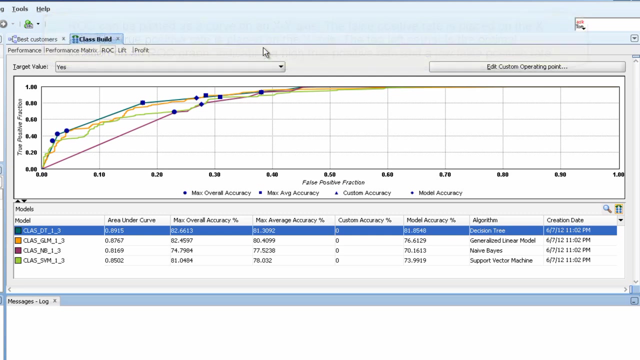 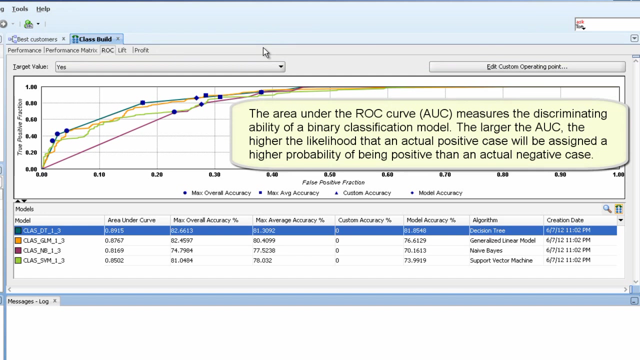 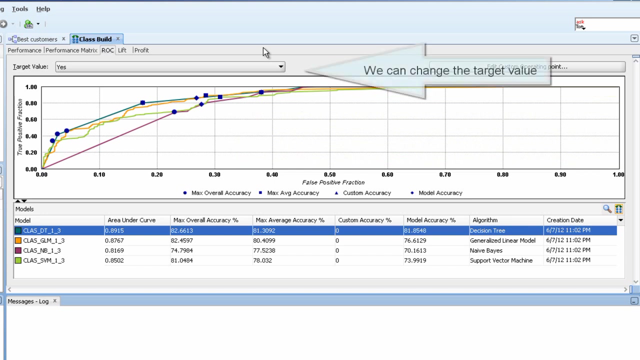 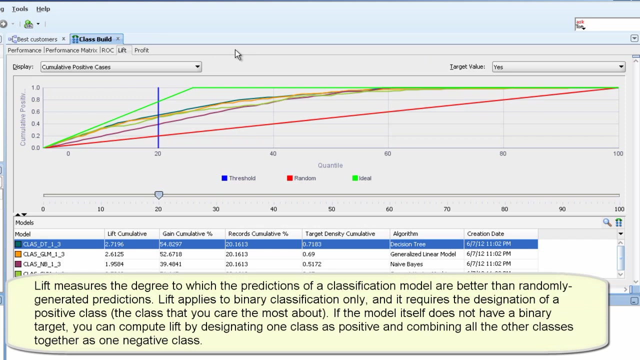 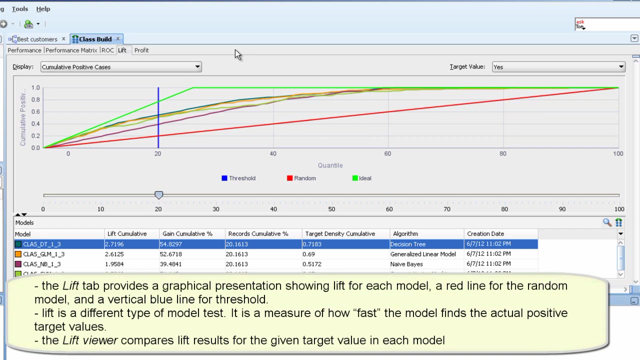 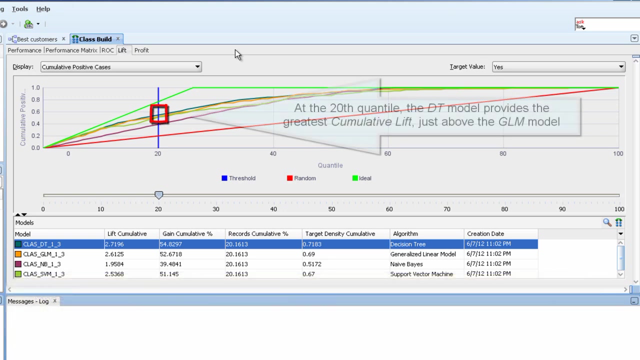 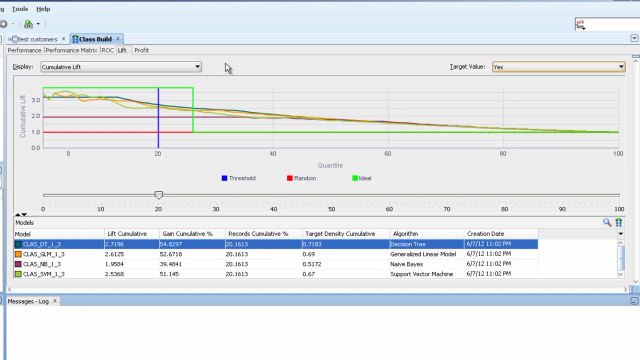 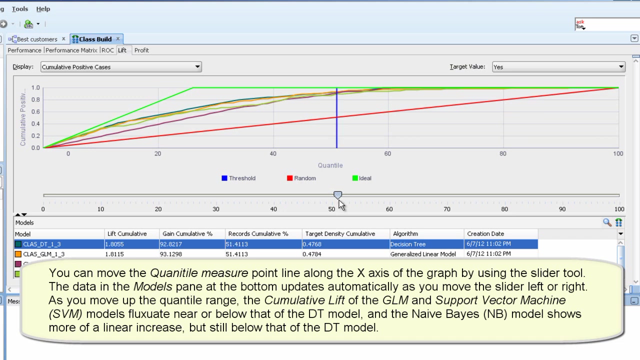 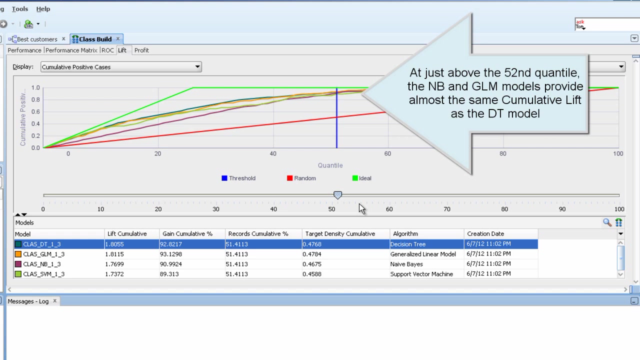 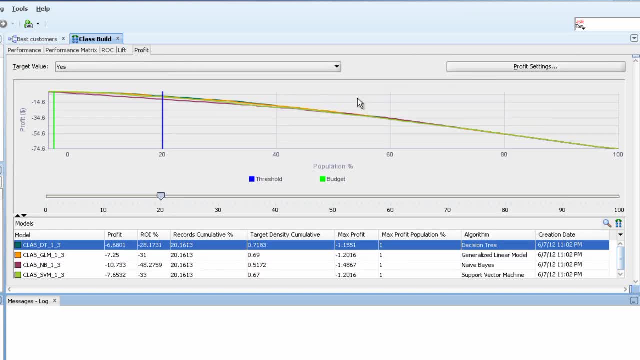 At just above the 50 second quantile. the NB and GLM models provide almost the same cumulative lift as the DT model. Preficient, motivation, Difficulty, Advertising, Consumers, Common methyl, magic Signs, Doors, lurid text, More infos. 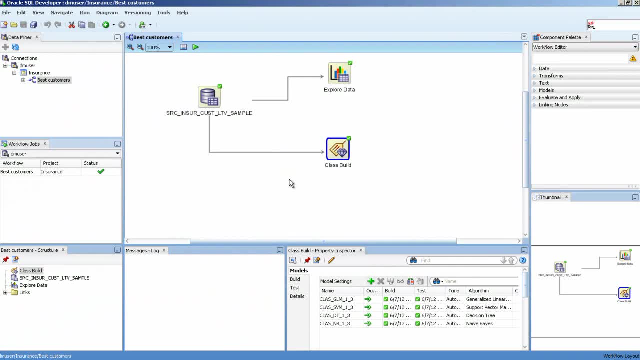 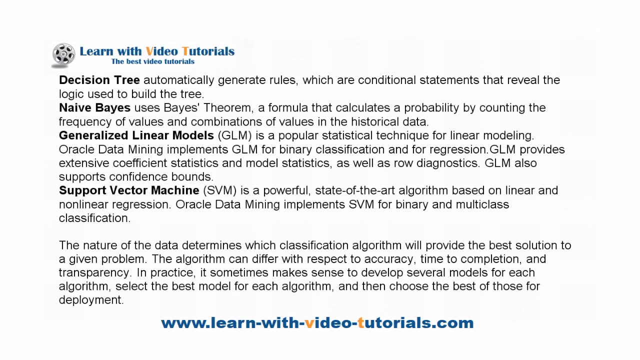 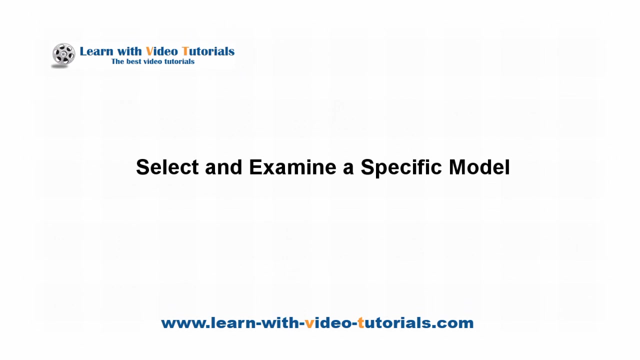 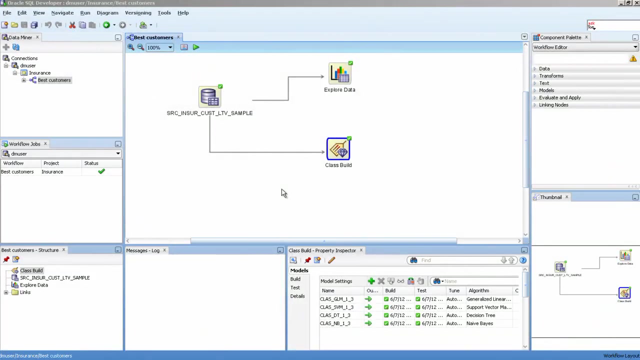 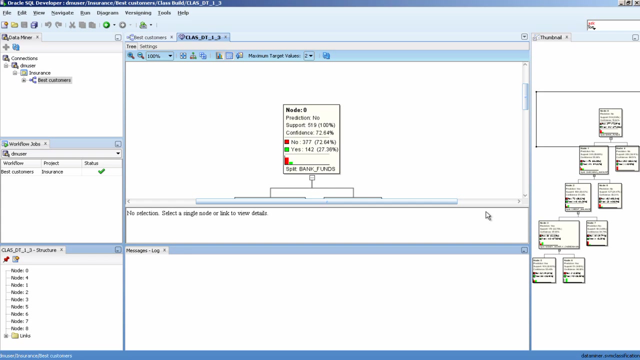 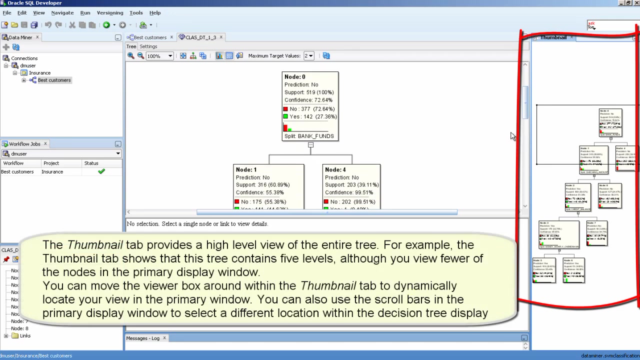 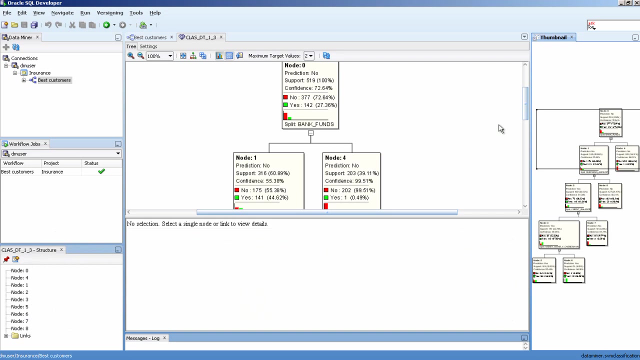 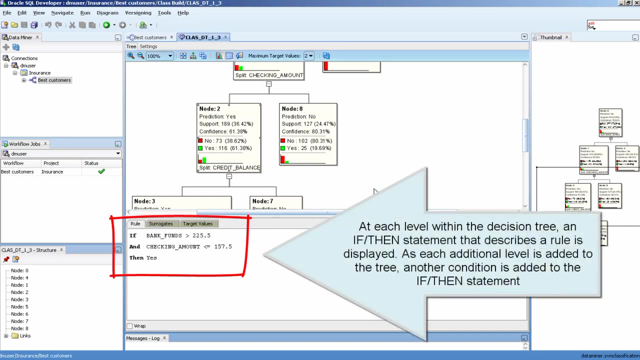 Here are some sign asian pictures. We'll be right back, Select and examine a specific model. Right-click the Class Build node again and select View Models, Class Details and OK. Click on Node 2 to select it At each level within the decision tree. 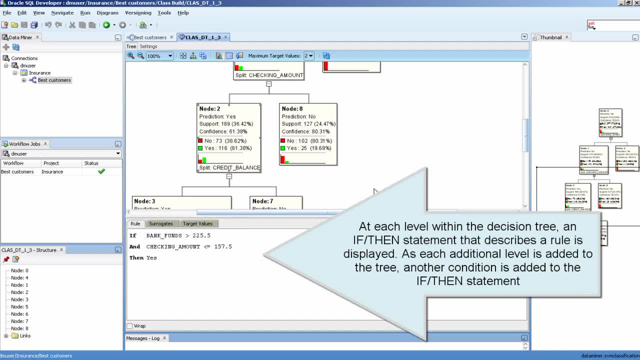 an if then statement that describes a rule is displayed. As each additional level is added to the tree, another condition is added to the if then statement For each node in the tree. summary information about the particular node is shown in the box. 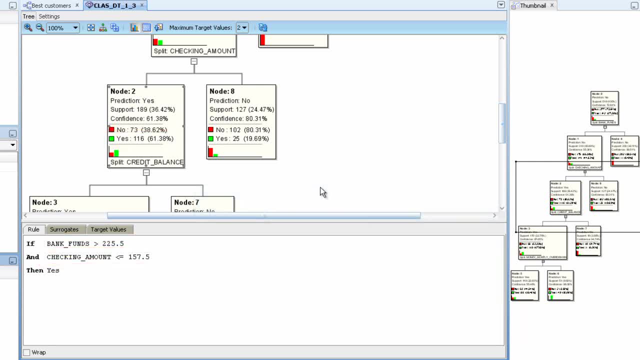 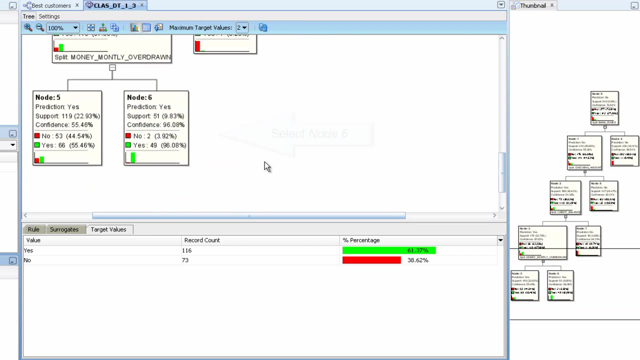 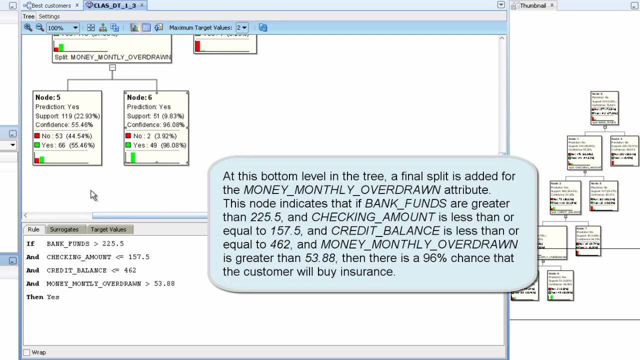 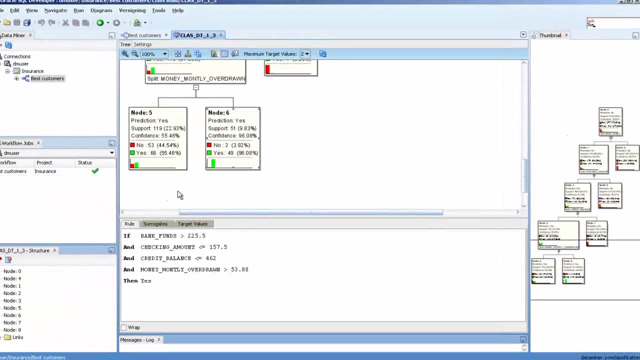 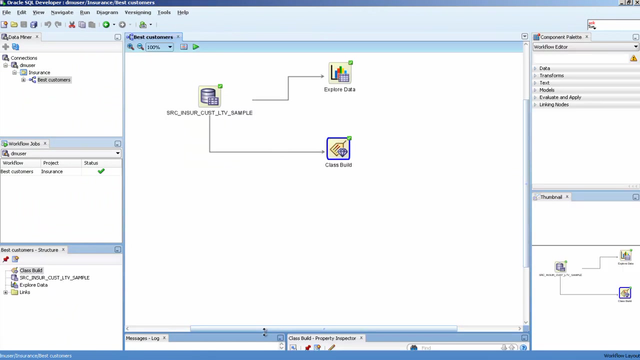 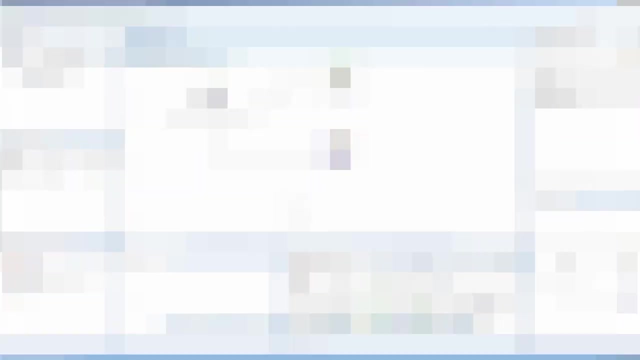 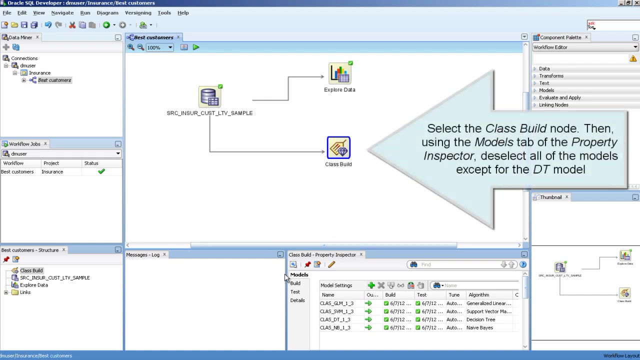 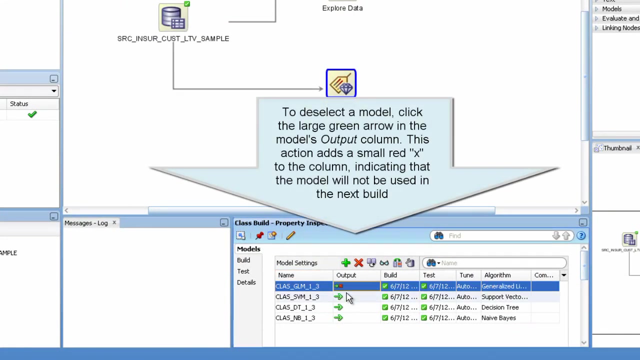 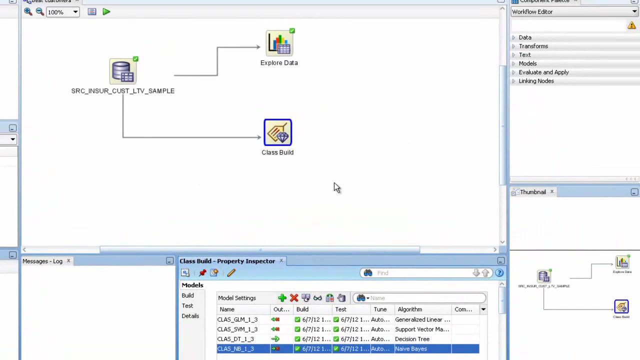 You will need to backs total. A surrogate rule is a related attribute that can be used at apply time if the attribute needed for the split is missing. Select node 6. Apply the model. Select the Class, Build node. Then, using the Models tab of the Property Inspector, deselect all of the models except for the DT model. 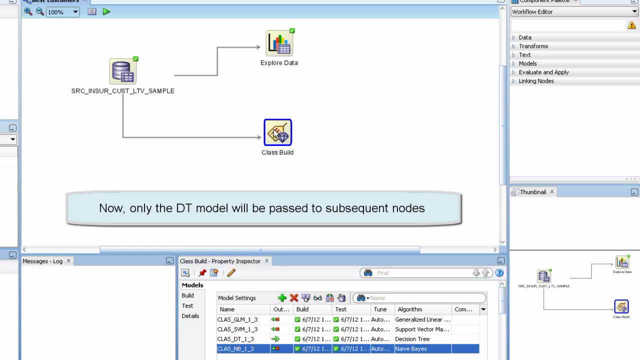 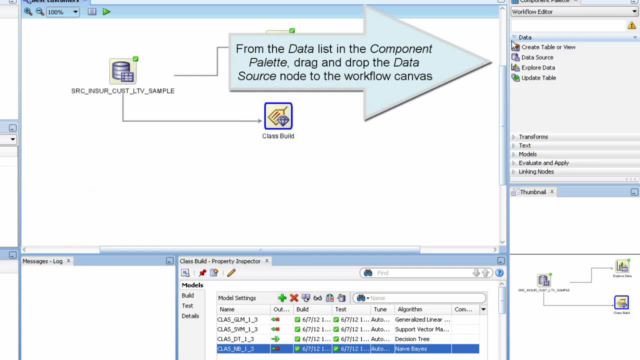 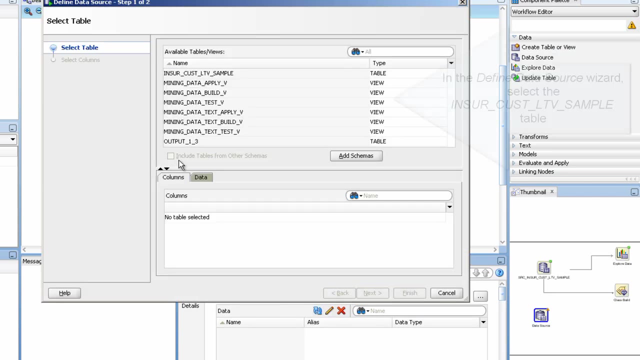 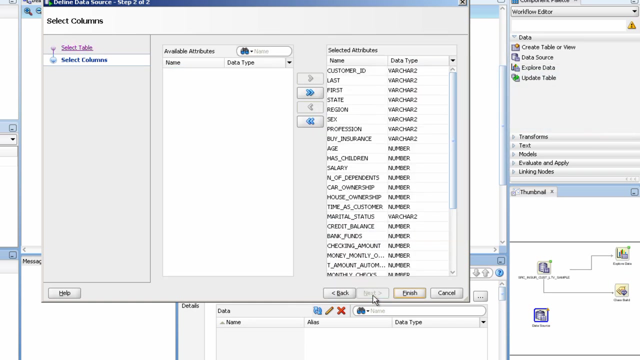 Now only the DT model will be passed to subsequent nodes From the data list in the Component palette. drag and drop the DataSource node to the Workflow canvas. In the defined DataSource wizard, select the InSuaCust LTV Sample table. 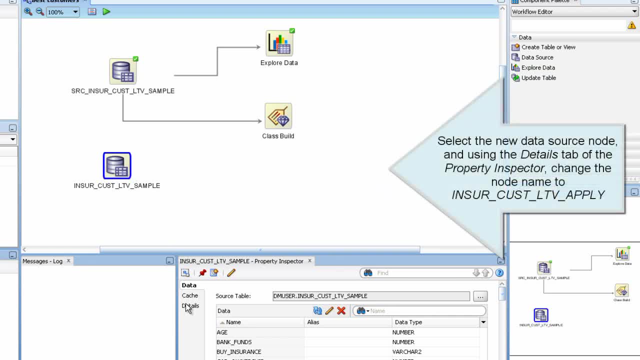 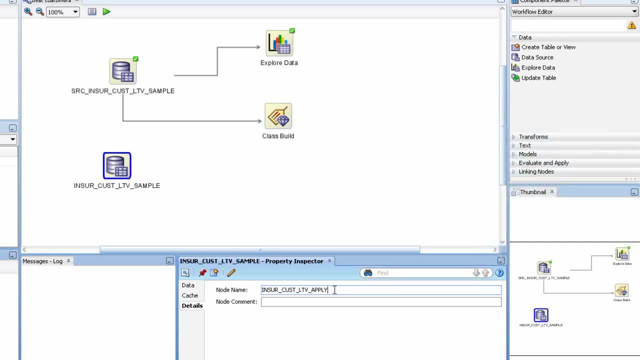 Select the new DataSource node and, using the Details tab of the Property Inspector, change the node name to InSuaCust LTV- Apply. The new table name is reflected in the workflow. Open the Evaluate and Apply list in the Components palette. 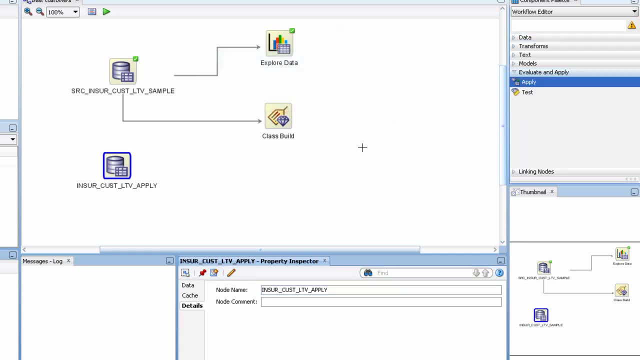 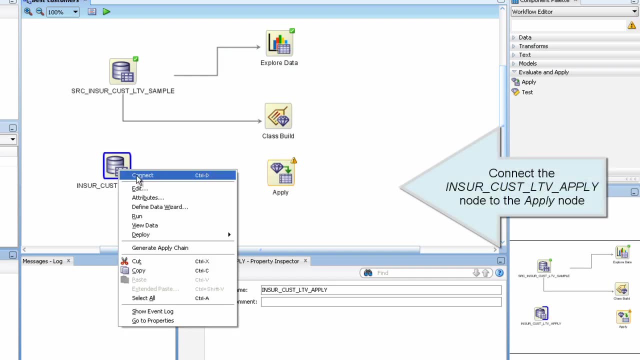 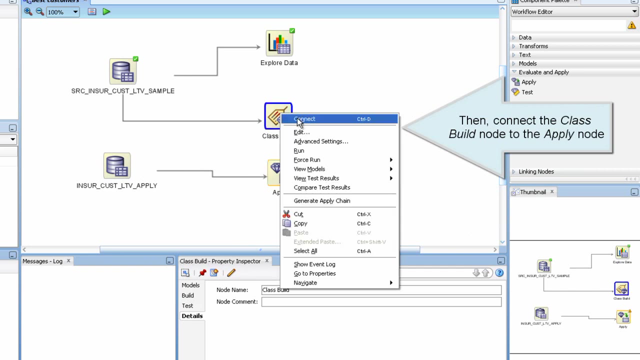 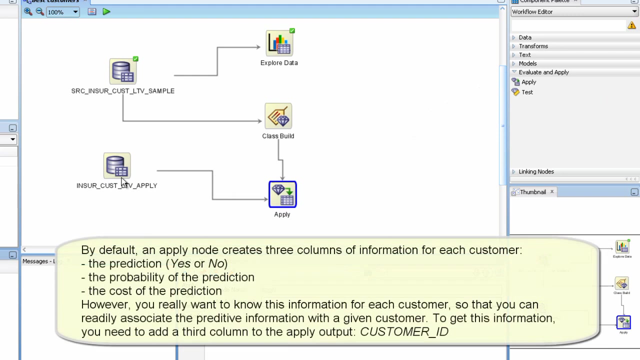 Next drag and drop the Apply node to the Workflow canvas. Connect the Source node to the Apply node Then connect the Class Build node to the Apply node. Connect the Class Build node to the Apply node, Then connect the Class Build node to the Apply node. 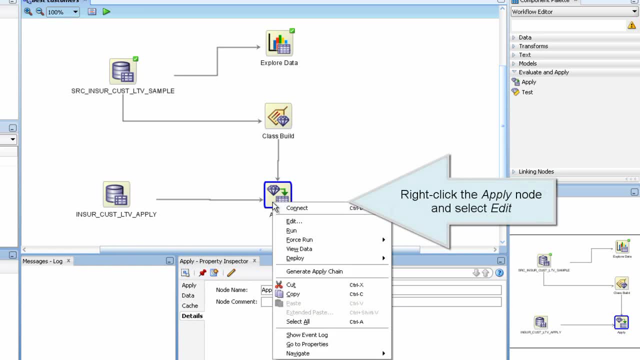 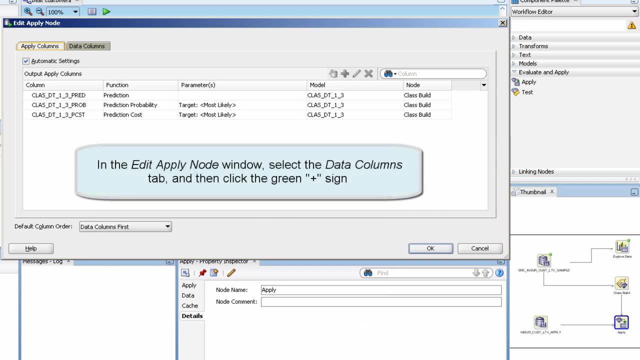 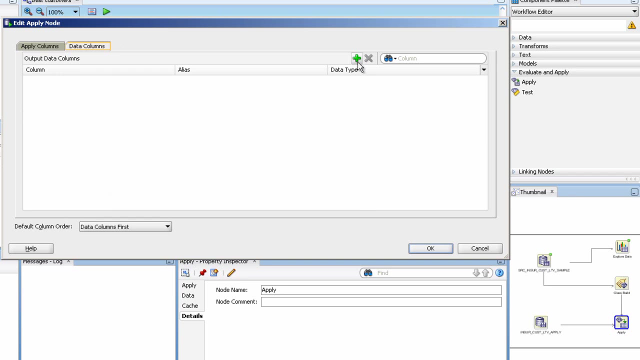 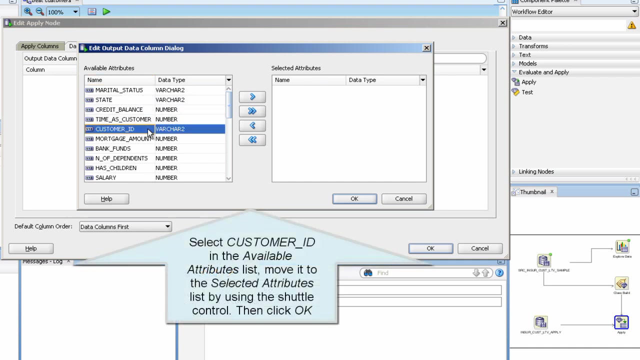 Right-click the Apply node and select Edit. In the Edit Apply node window, select the Data Columns tab and then click the green plus sign. Select Customer ID in the Available Attributes list. move it to the Selected Attributes list by using the Shuttle control. 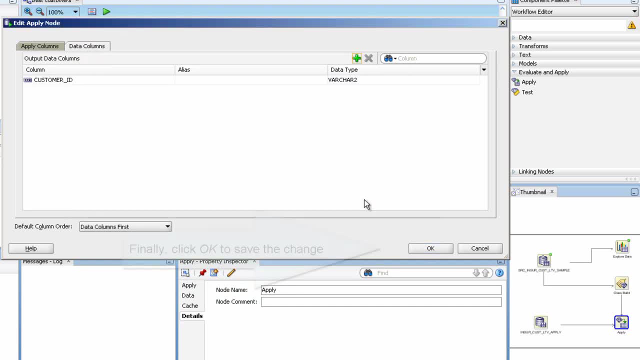 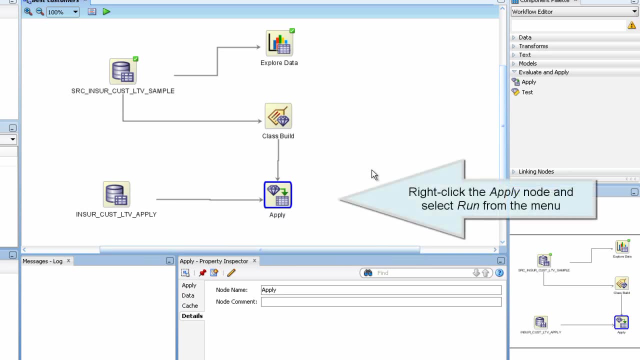 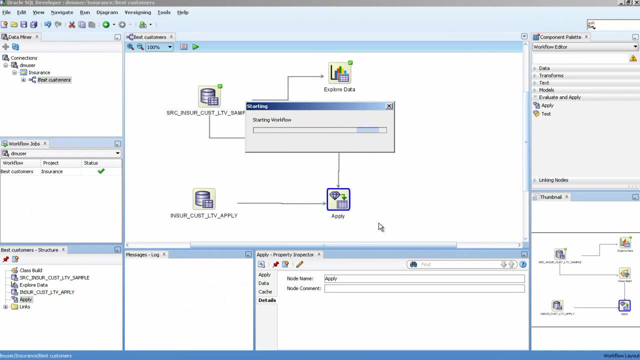 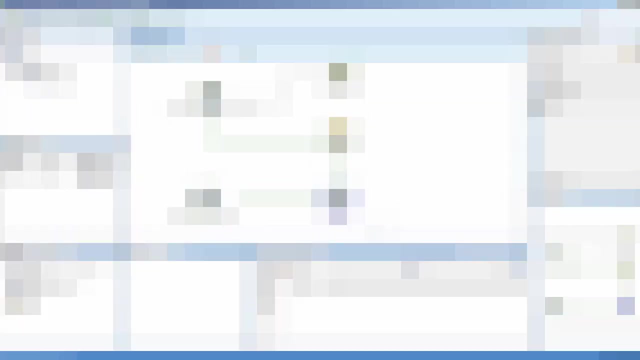 Then click OK. Finally, click OK to save the change. Right-click the Apply node and select Run from the menu. You can だん may enter the OK distribution of the configuration by selecting the right and left section of the menu and click the Now button. 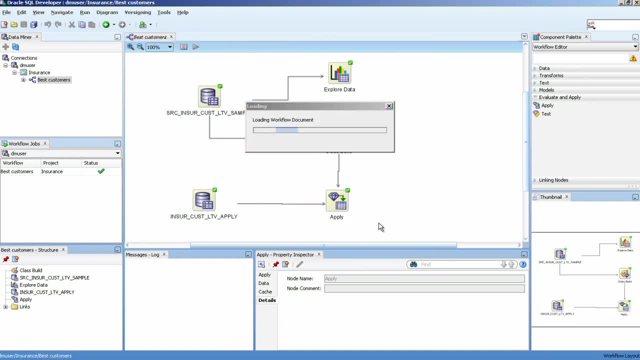 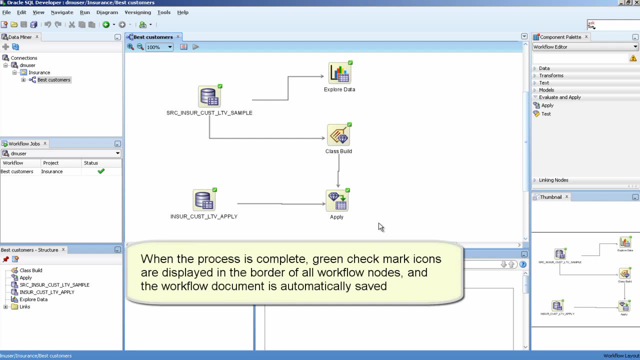 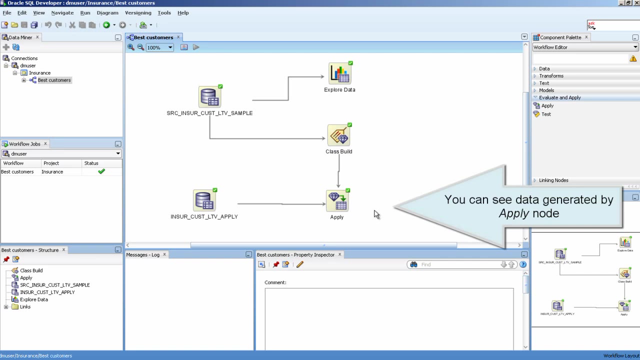 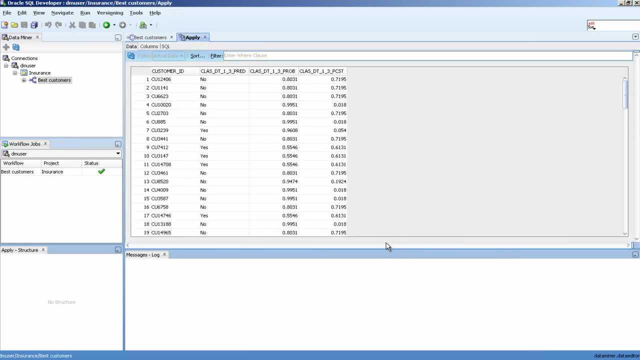 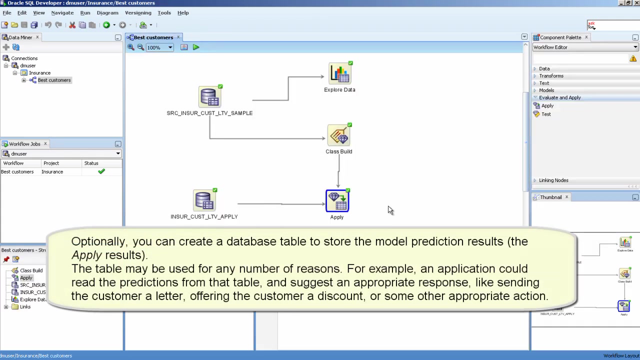 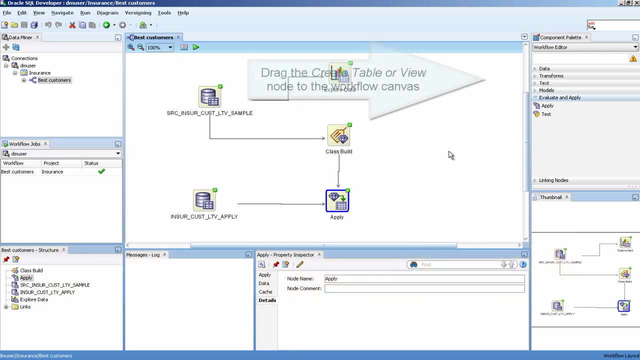 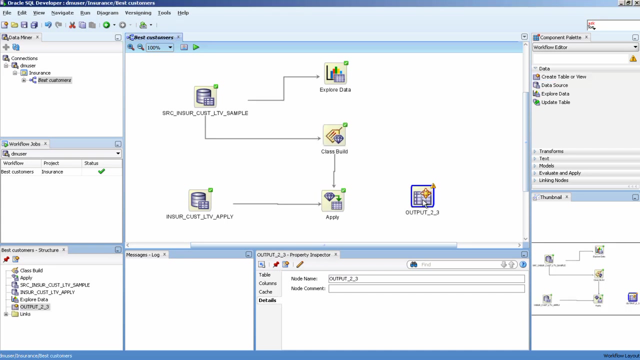 Thehet will be available in. You can see data generated by apply node. Drag the create table or view node to the workflow canvas. Drag the create table or view node to the workflow canvas. Drag the create table or view node to the workflow canvas. 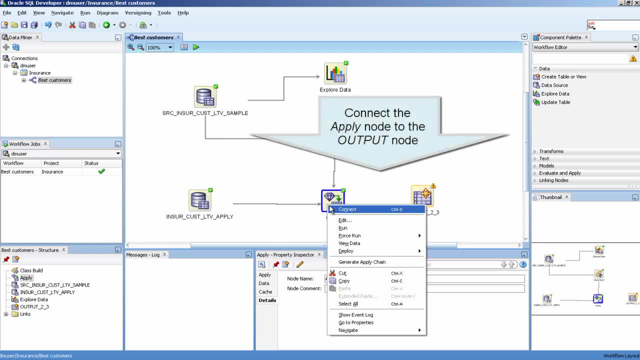 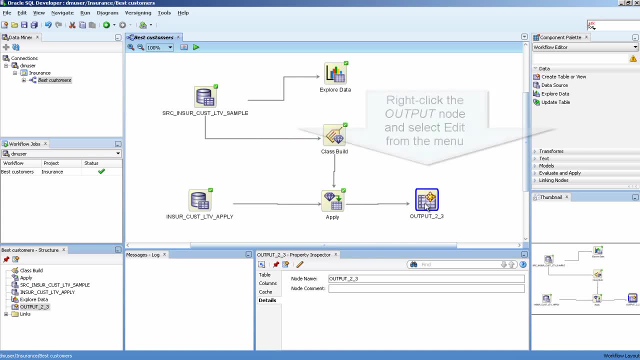 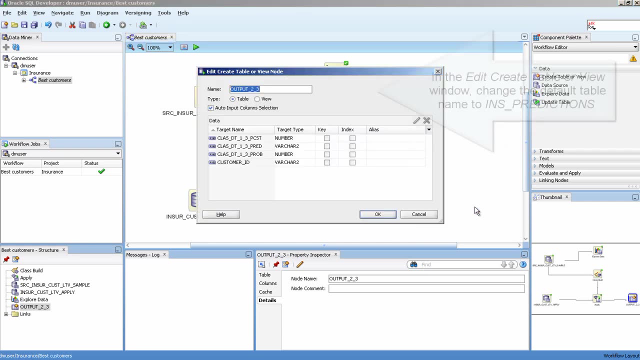 Connect the apply node to the output node. Right click the output node and select edit from the menu. In the edit creator, select the output node. In the edit creator, select the output node. In the edit creator, select the output node. 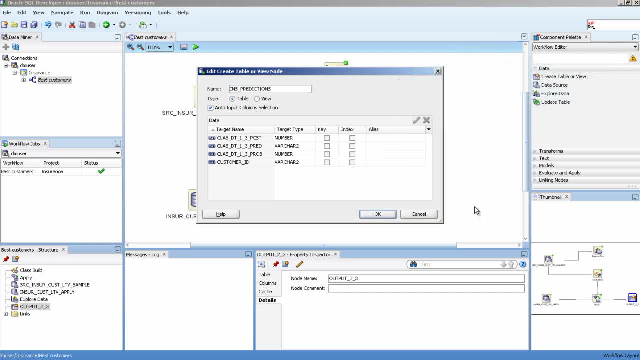 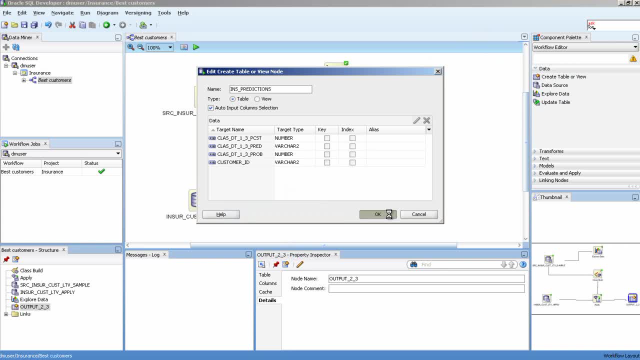 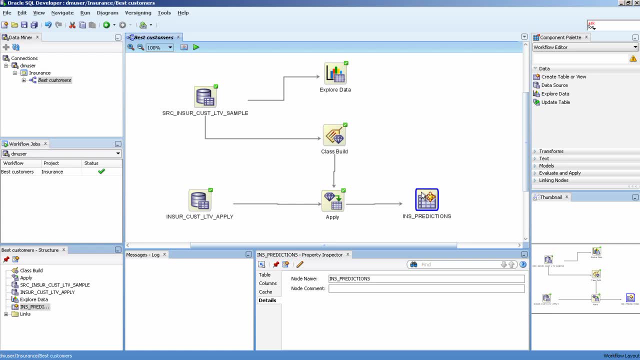 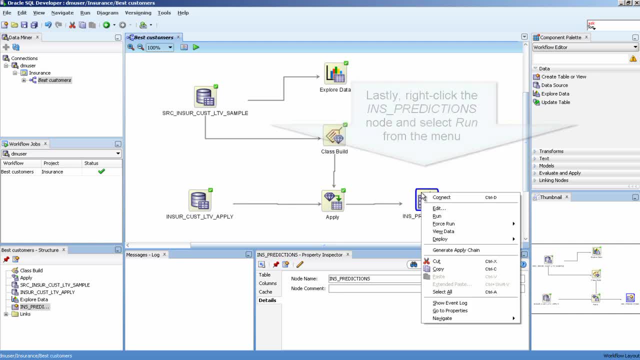 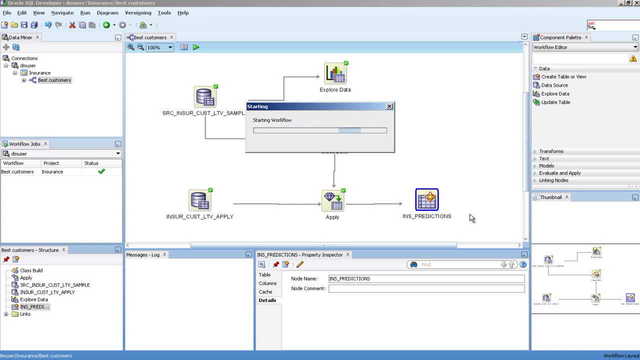 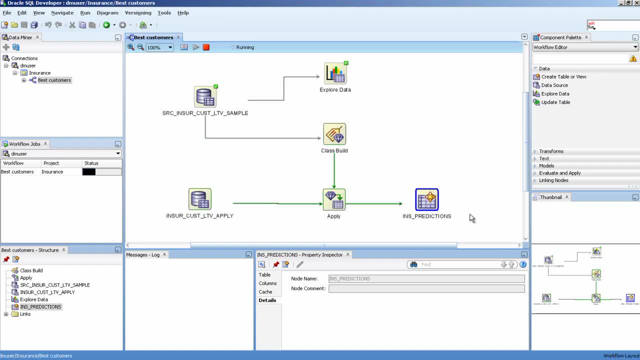 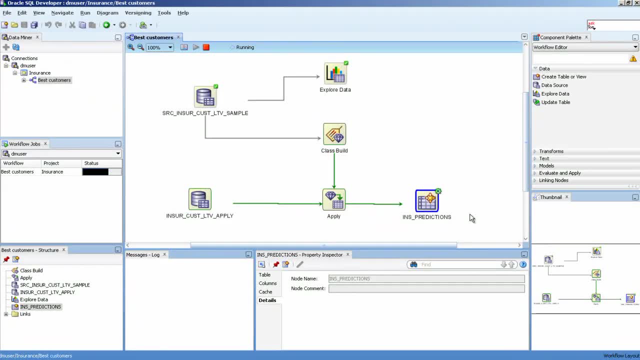 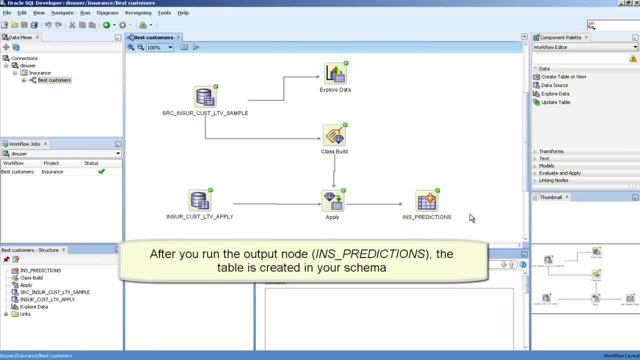 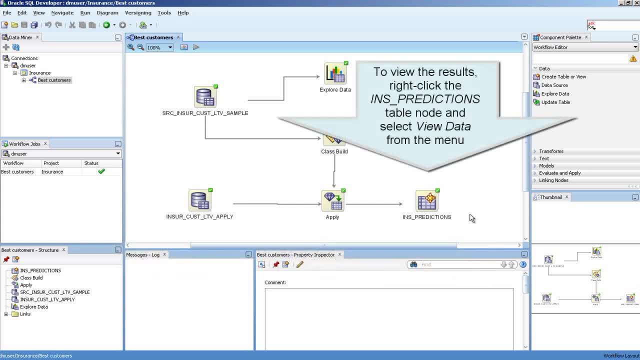 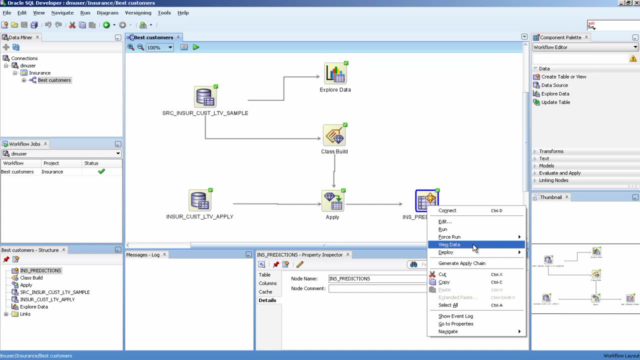 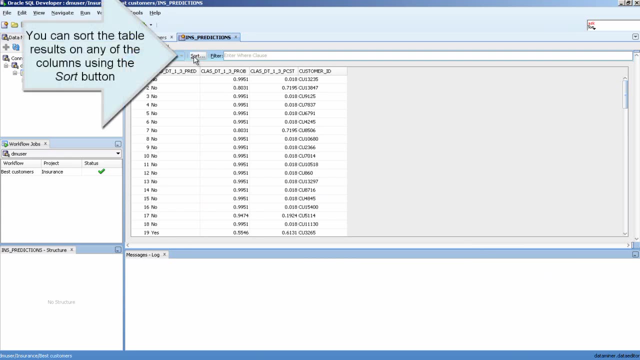